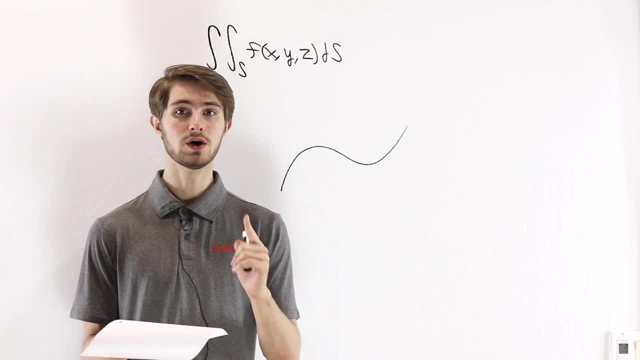 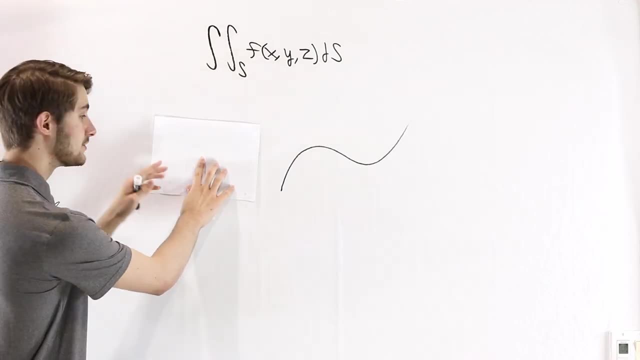 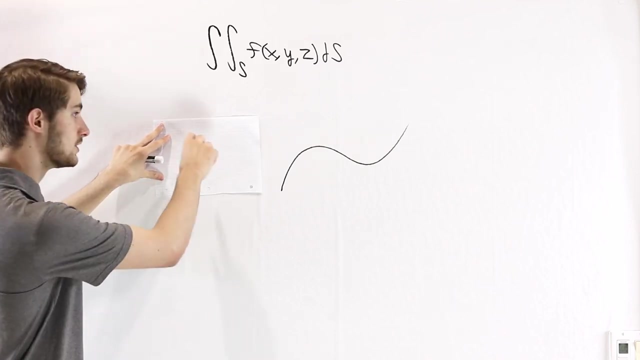 Now, if it's difficult to think about a shape in four dimensions, one way you can think about the surface integral is that we first take our surface in three dimensions and flatten it so that it exists only in two dimensions, From there evaluating the function at every point on the surface. 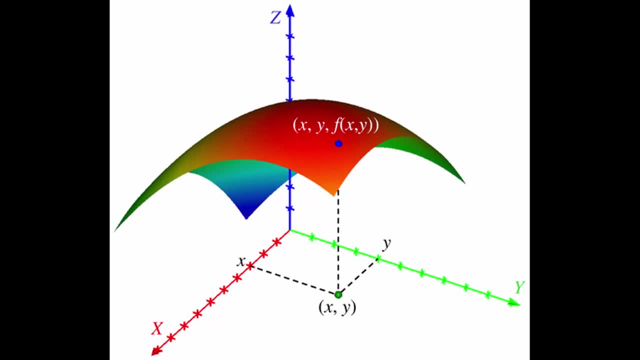 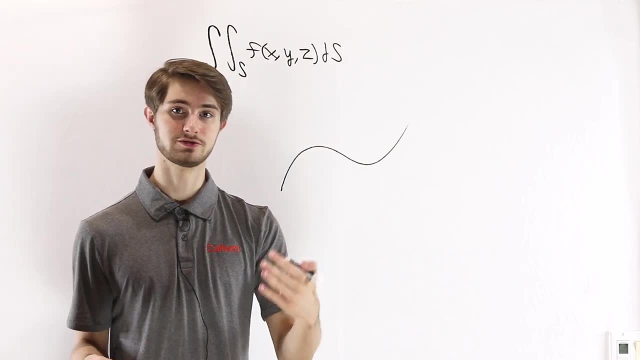 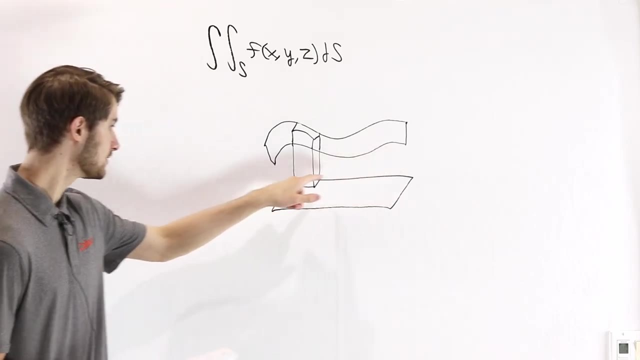 corresponds to giving this a height. So we're just looking at an ordinary three-dimensional function on top of this surface and we take the volume That would be our surface integral. Remember that when we were doing ordinary double integrals we would consider a two-dimensional input region. 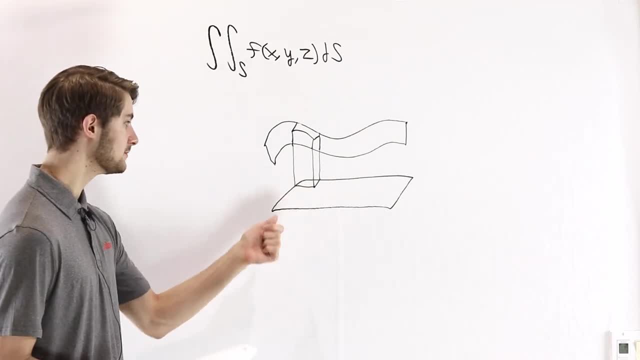 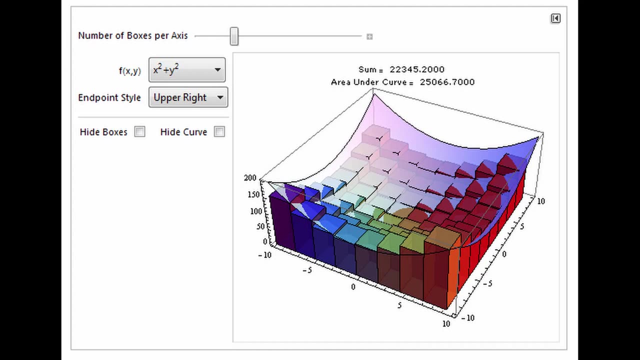 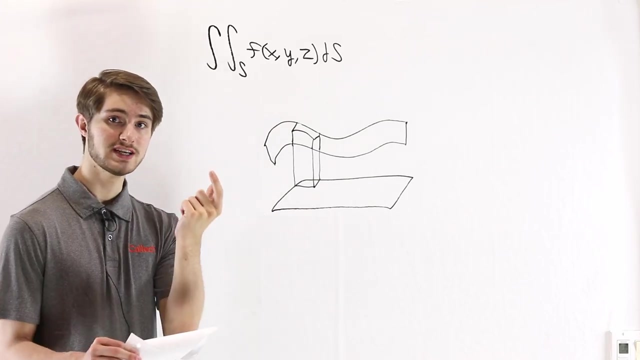 and the way that we computed the integral was by first splitting that region into a bunch of rectangles. We use those rectangles as the base and then we would take the height to be the function evaluated at each point. so this becomes a three-dimensional idea. Then that one small part. 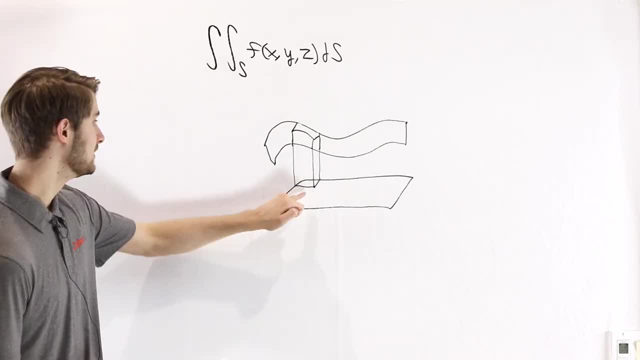 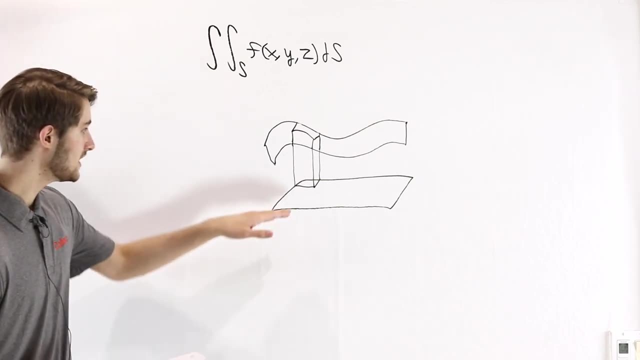 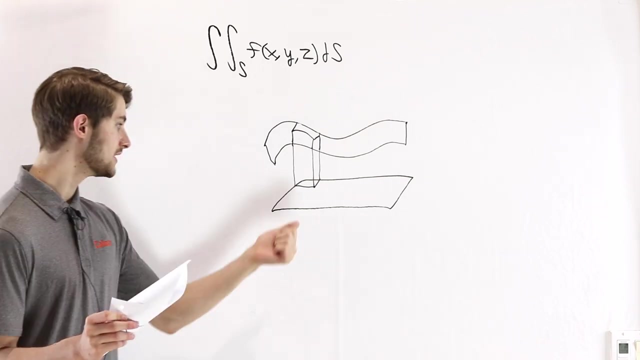 of the integral is the volume of this rectangular prism, the base times the height. When we're doing a surface integral, we're looking at the same idea, but instead of looking at a two-dimensional input region, our input region is a surface in three dimensions and therefore, instead of just 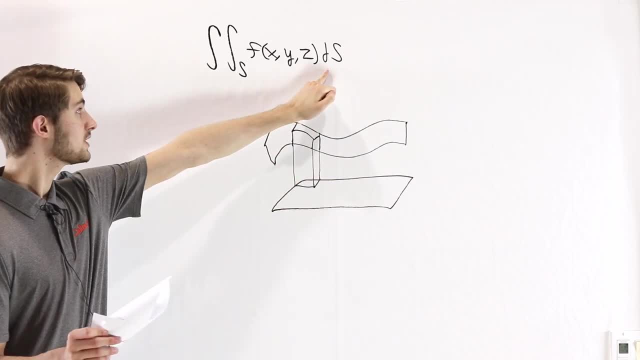 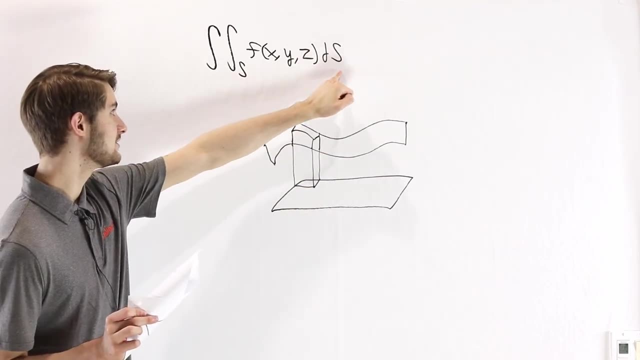 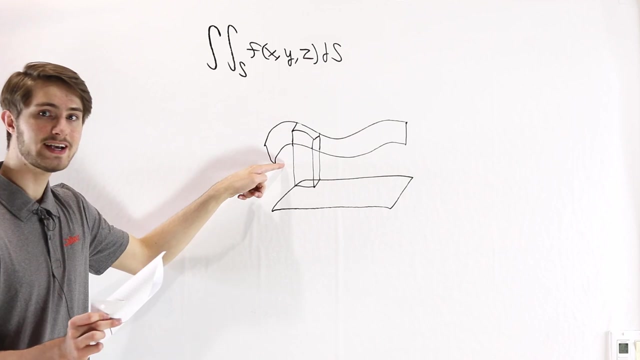 looking at a change in area along this region. we're looking at an area on this surface and we call the area of a small region on this surface ds. So this expression here is saying that we take the function evaluated at some point on the surface. that's the height of this rectangular. 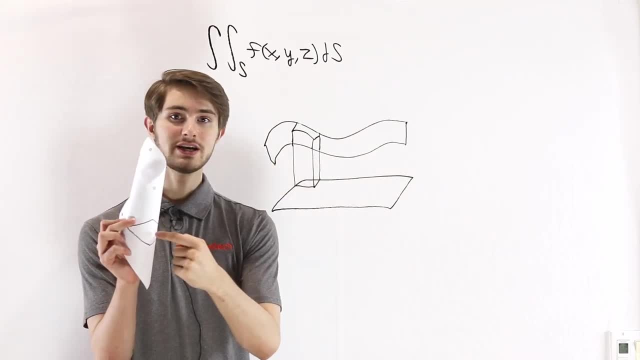 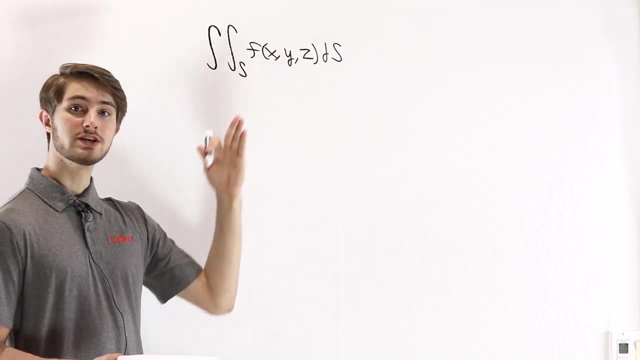 prism, and then we multiply by the base, which is the area of a small part of this surface ds. So now that we have this expression for a scalar field, surface integral, we need to figure out a way to actually compute it, and the first step to doing that 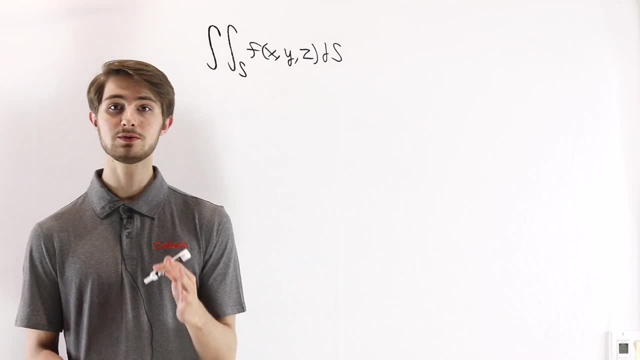 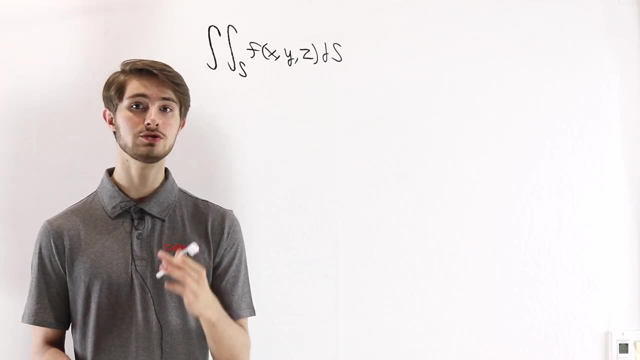 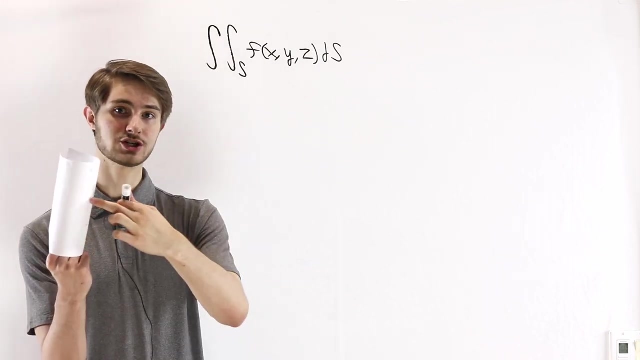 is understanding how to describe our surface. The way that we accomplish that is through a parametrization. Now, in order to parametrize a surface, we need to have two different variables, and the reason for that is that with the surface, there are two different independent directions. 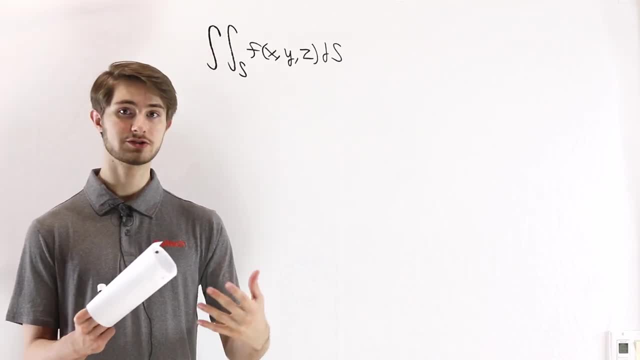 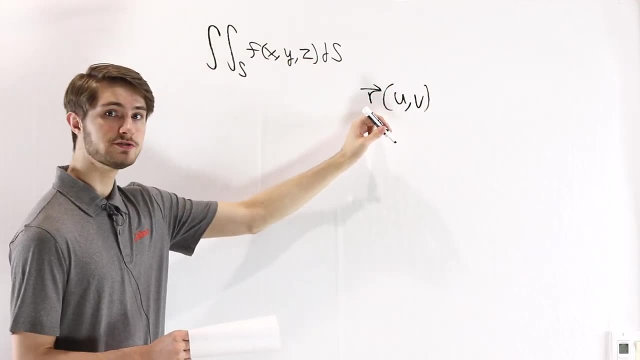 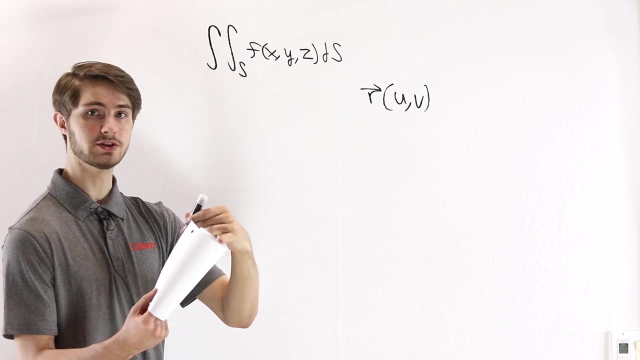 of movement. So in order to describe every point on the surface, we need to have a parametrization in terms of two variables. So we have a vector-valued function, r of two variables- u and v- that takes in these two variables and outputs a point on the surface. Then we can describe. 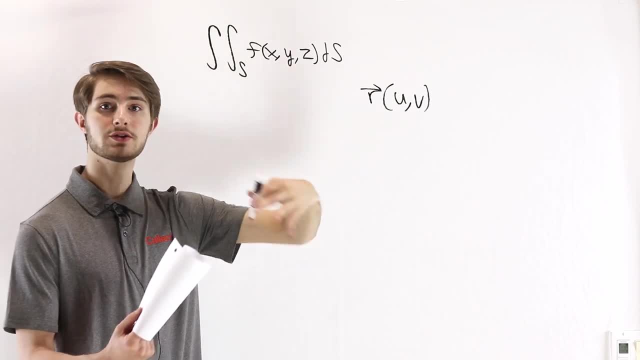 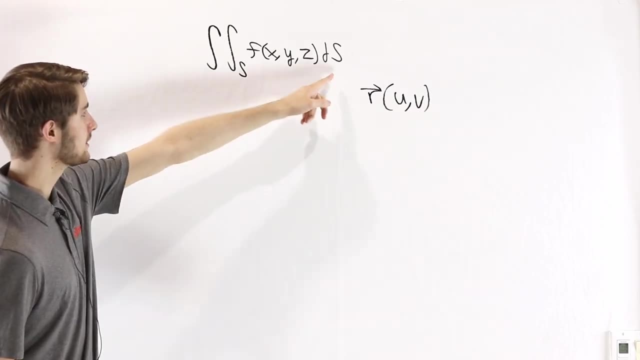 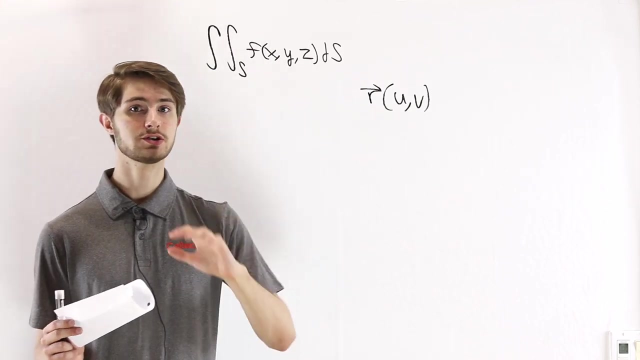 the range of values u and v that gives every point on the surface we're interested in. Now that we have this parametrization r of u and v, we can start to think about the how to calculate ds. Remember that ds is an area of a small section on the surface. 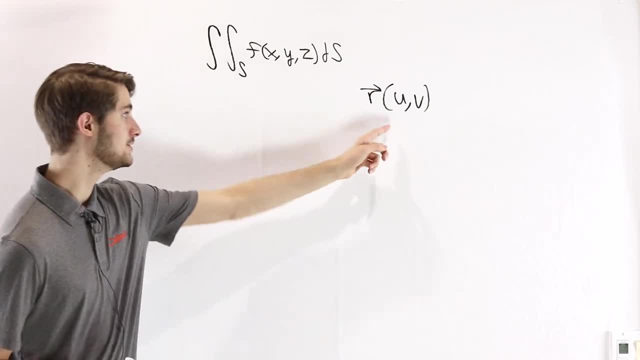 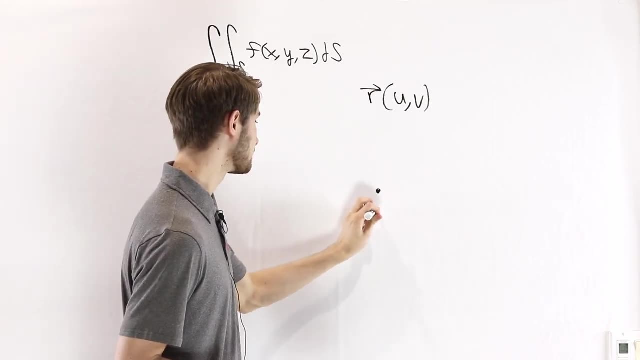 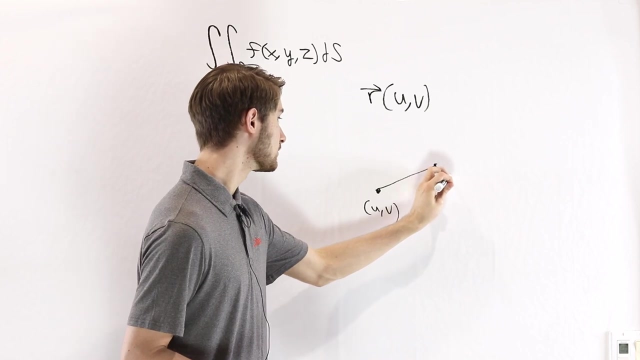 so we need to think about how we can represent that in terms of u and v. Remember that r of u and v is going to give us a point on the surface. If we change the value of u by some small amount, so that we're looking at u plus du instead, that's going to create a particular movement. 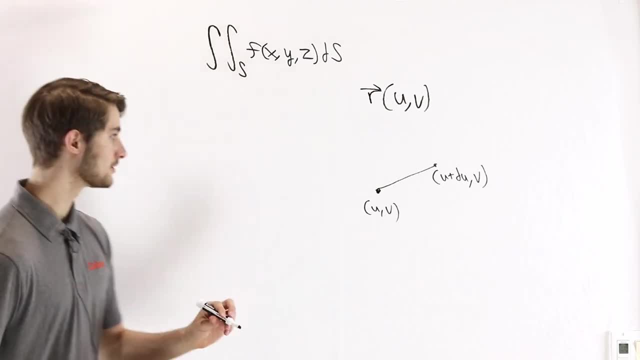 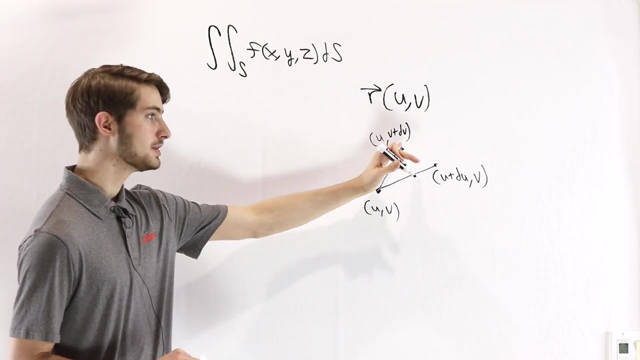 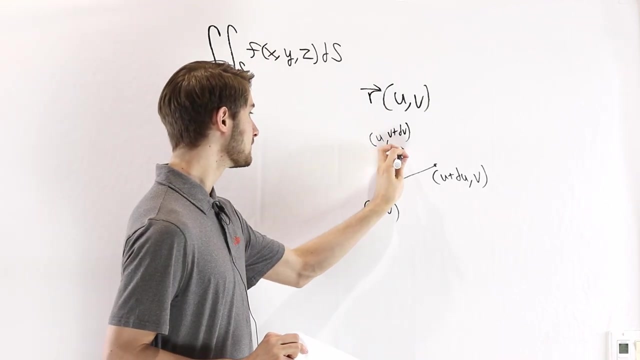 on the surface a movement in some direction. Similarly, if we do a small change in the value of v, so that we're looking at v plus dv, that's going to create a movement along this surface in a different direction. We can complete this picture by connecting to the final point u plus du. 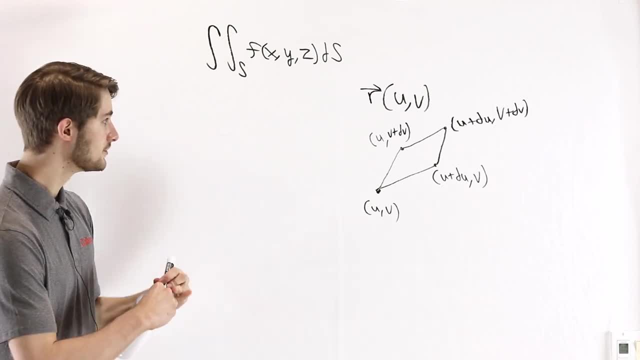 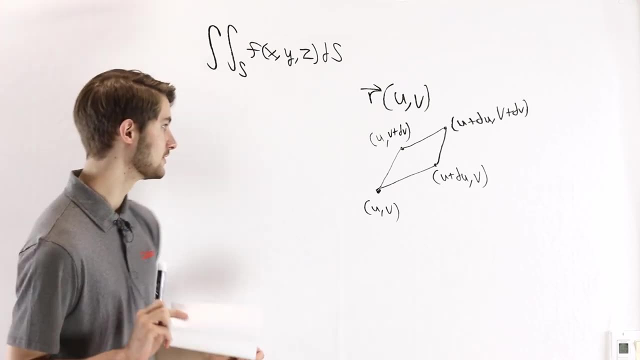 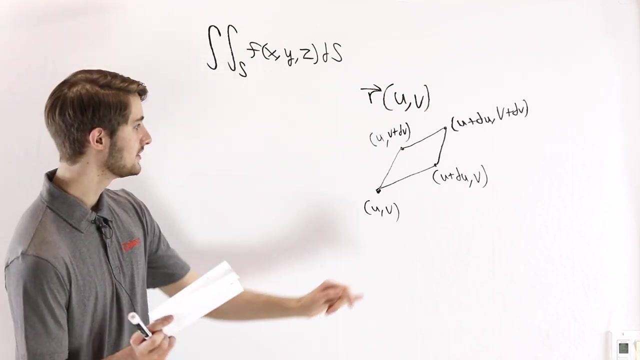 comma v plus dv. This area represents a small range of u and v values and how they map onto the surface. We want to find the area of this part of this surface. One important element of this calculation is that as we make du and dv very, very small, we can approximate the area. 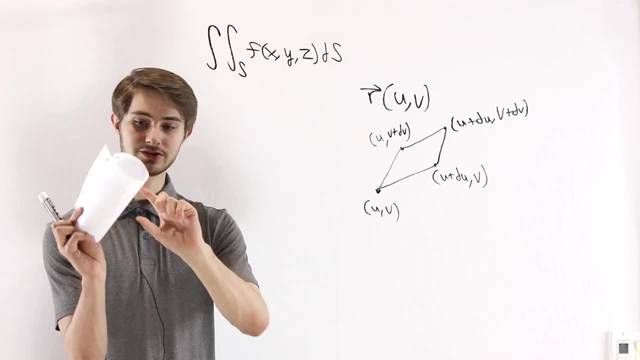 on this surface as a parallelogram. That's because as we get smaller and smaller ranges on the surface, we are bring along norms in parallelogram. They now appear very close to each other together and i'll just show you so you know a couple things about between per sec and one sec. Let's to the mean to become. 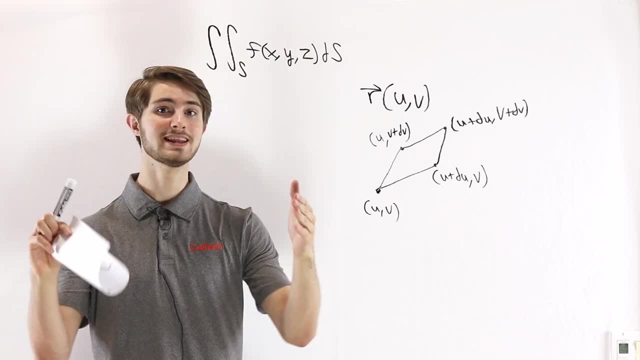 that at any time we get a smaller and smaller range of dv, heavier that it sociallyларger you're going to surface, we can start to approximate it as flat in that small region and therefore we're just looking at a parallelogram. 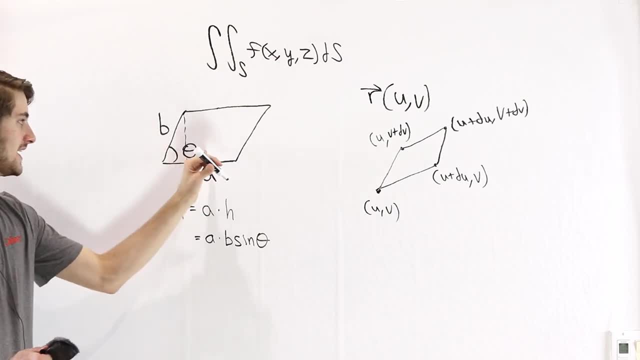 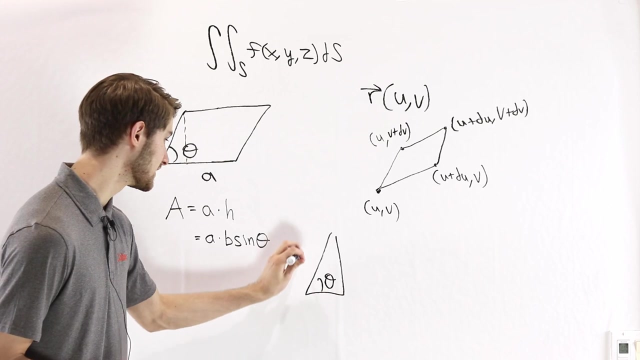 If we're looking at a parallelogram with side lengths a and b and an angle of theta between those two sides, the area is going to be the base times the height. but we can write the height in terms of b sine theta by looking at a right triangle just like this, where we 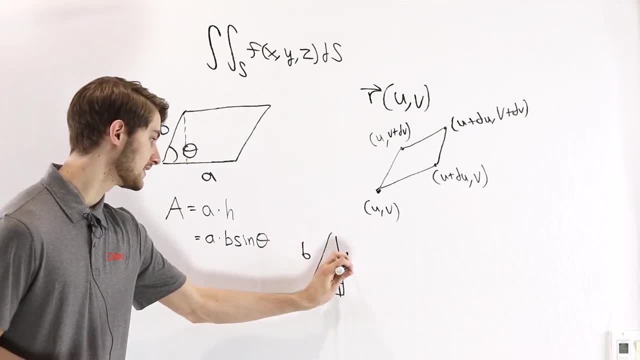 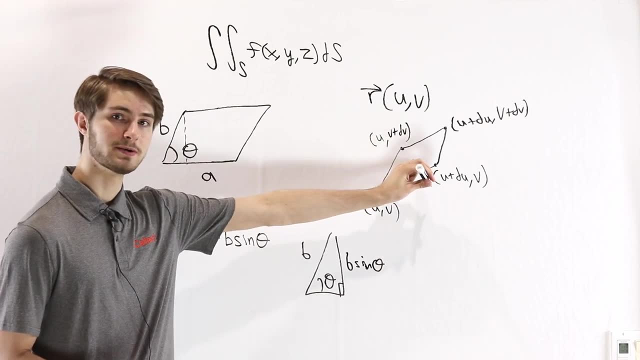 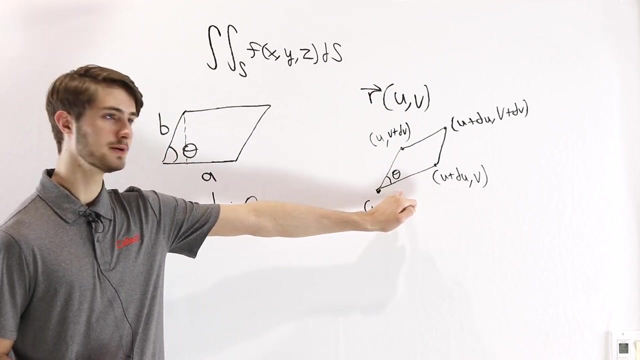 have the side b as the hypotenuse, then b sine theta becomes this side. We can use this formula to find the area of our parallelogram over here. To use this formula, the first step here is to find the side lengths of these parallelograms. 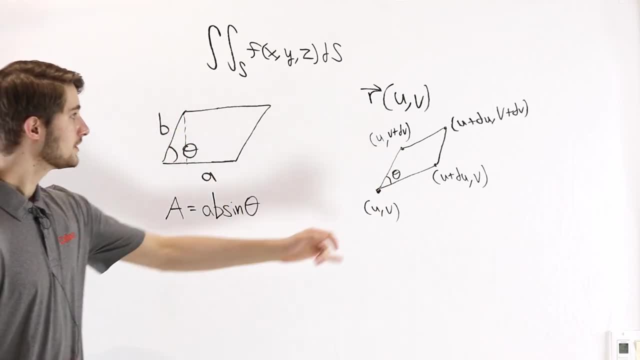 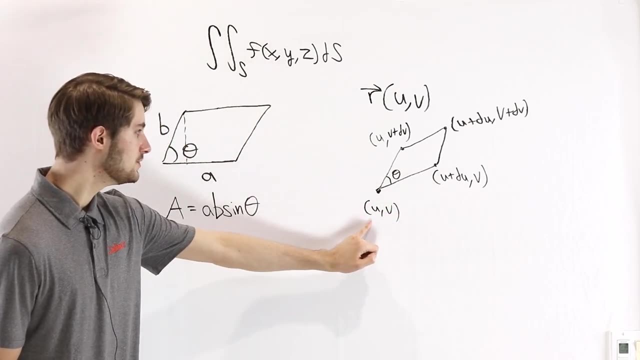 Remember that each of these sides represents a movement purely due to a change in one variable. Along this side, we aren't changing v at all. we're only moving in the direction of the parallelogram. We're only moving in the direction of increasing u from u to u plus du. 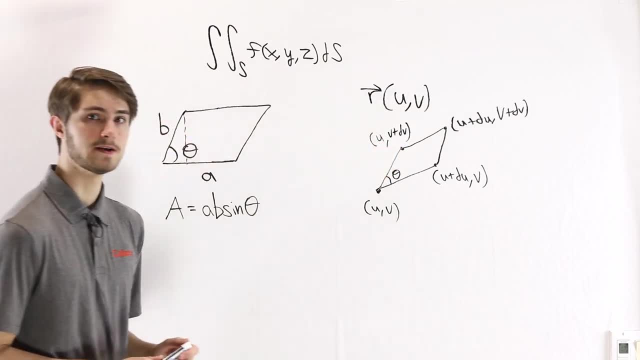 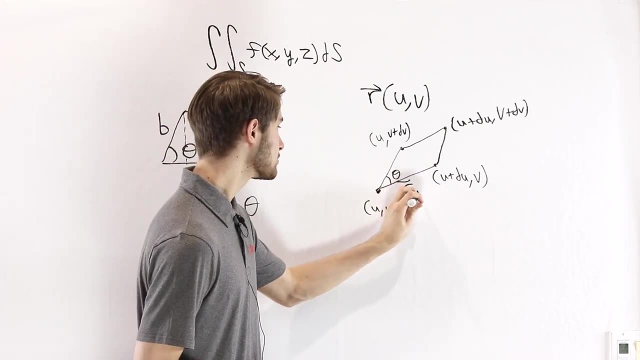 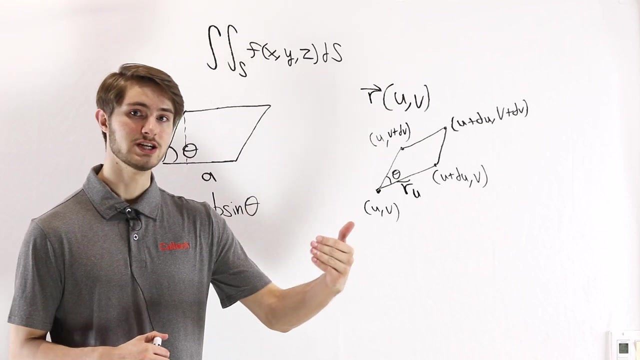 If we're looking at a vector-valued function, r of uv, the movement caused by a small change in u is going to be in the direction of the partial derivative of r with respect to u. That partial derivative represents. how does r change as we change u? and that's the direction. 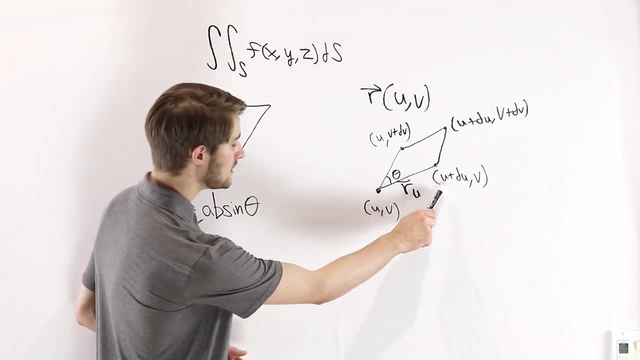 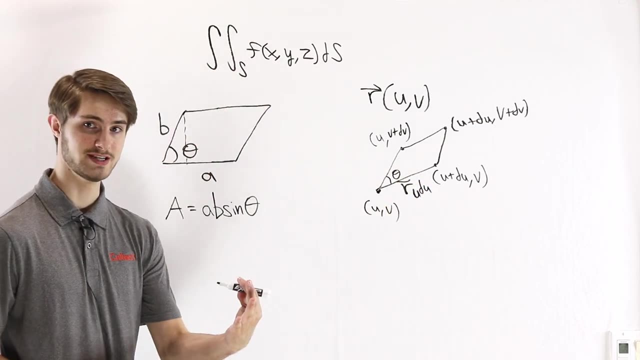 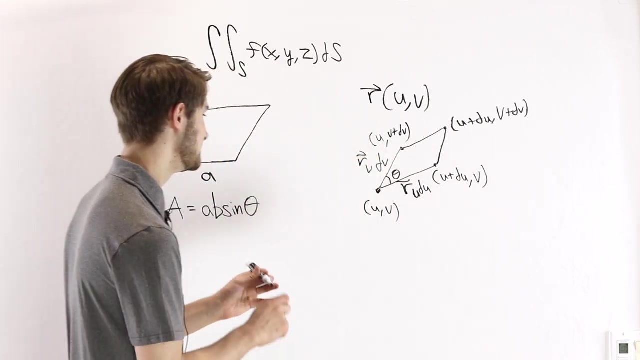 we're looking for And if we want that change in terms of a small movement du, the length of this side is going to be r sub u times du. Similarly, the side length up here is going to be r sub v times dv. 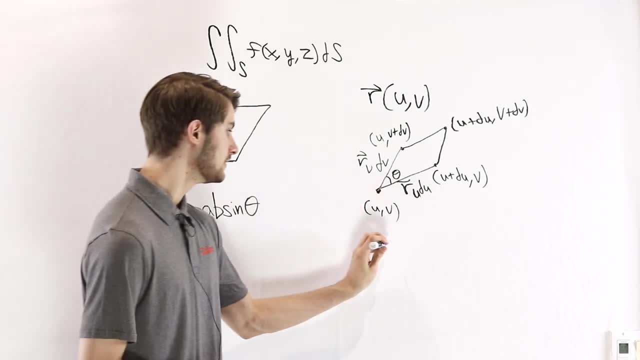 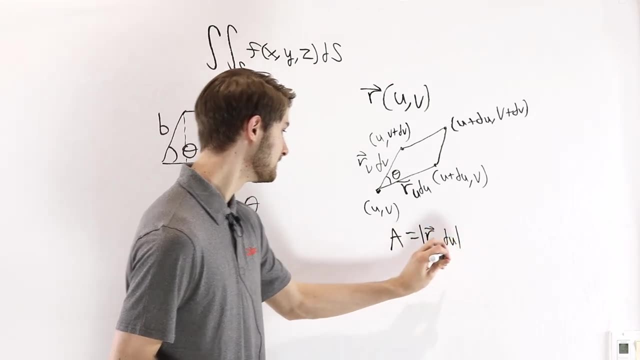 And from here we can start plugging things into this formula. The area is going to be the length of this side, which will be the magnitude of r sub u times du times the length of this side. the magnitude of r sub v times dv. 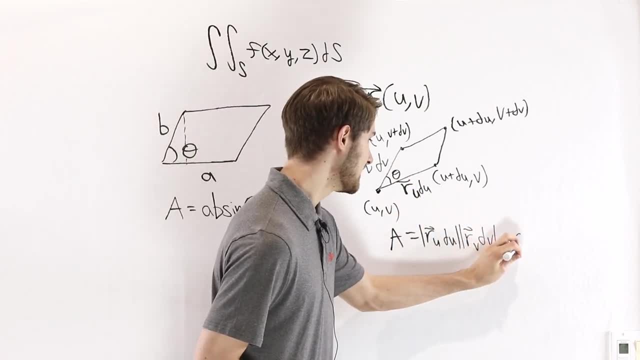 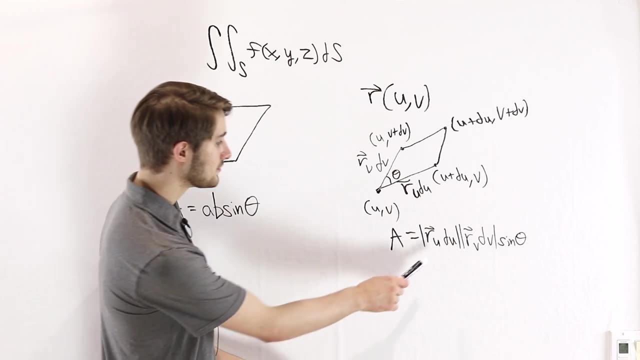 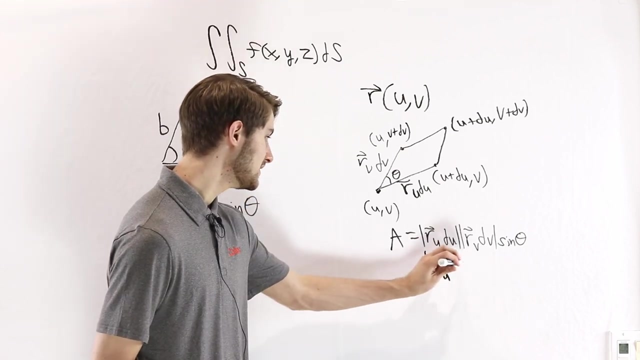 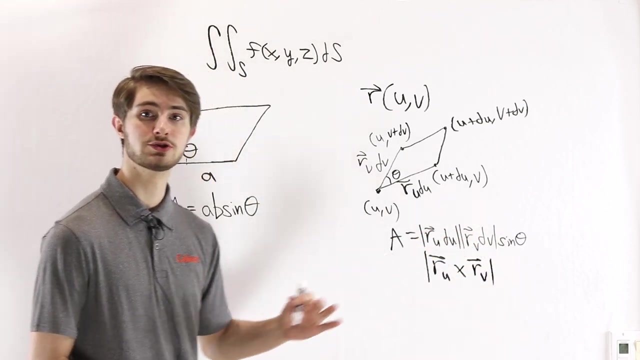 This formula is actually something that we've studied before. It is the formula for the magnitude of the cross product, the cross product between these two vectors, r sub u and r sub v. Here, because du and dv are both just scalars, I'm going to factor them out of that cross. 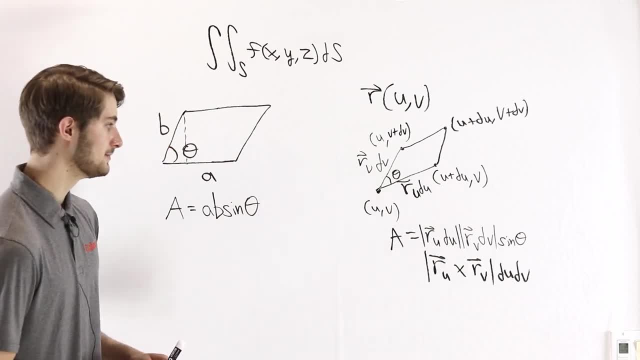 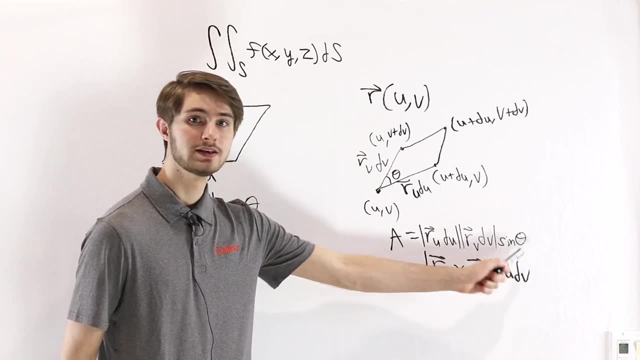 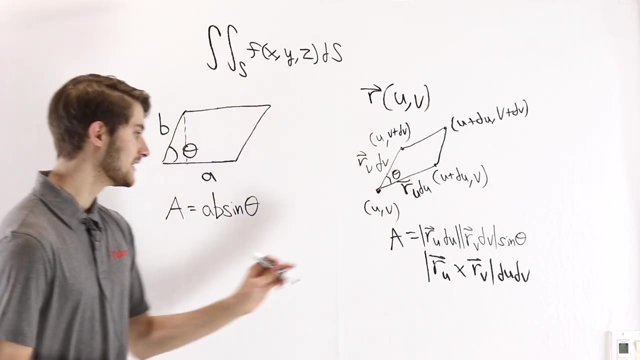 product. So, because the area of this parallelogram is given by the magnitude of the first vector times, the magnitude of the second vector times, sine theta, that expression is just the magnitude of the cross product. So the area of this parallelogram ds is equal to the magnitude of r sub u cross r. 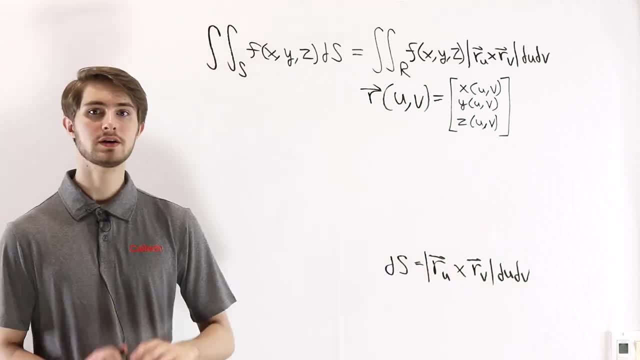 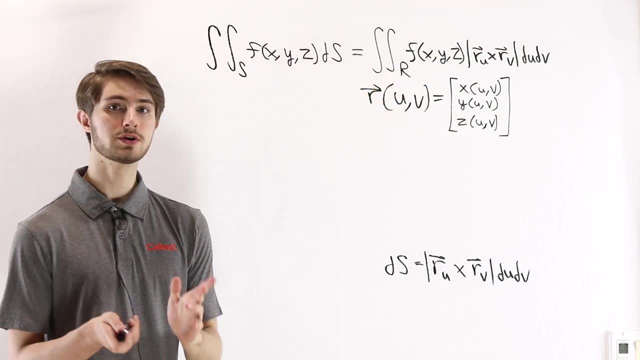 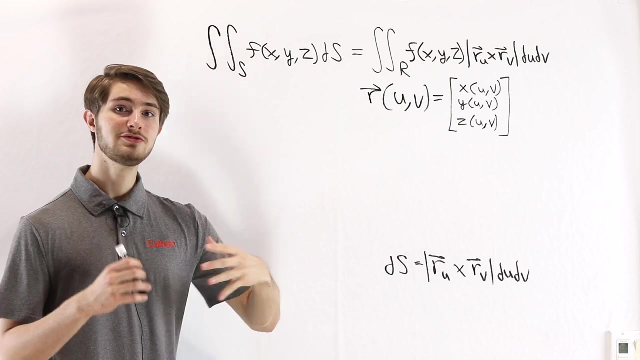 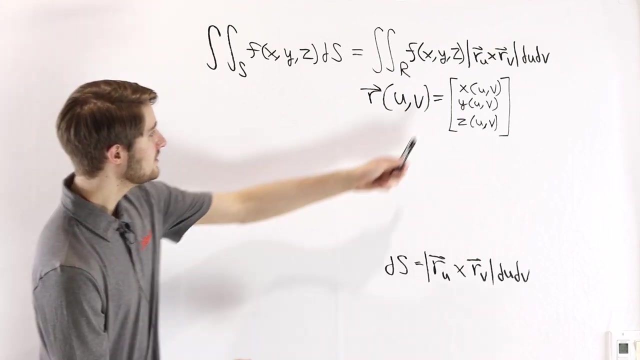 sub v times du dv. Now we can plug this formula for ds into our original surface integral. In this case, r is talking about the range of uv values that describe our entire surface And because r of uv, our parametrization gives the x, y and z values on the surface. 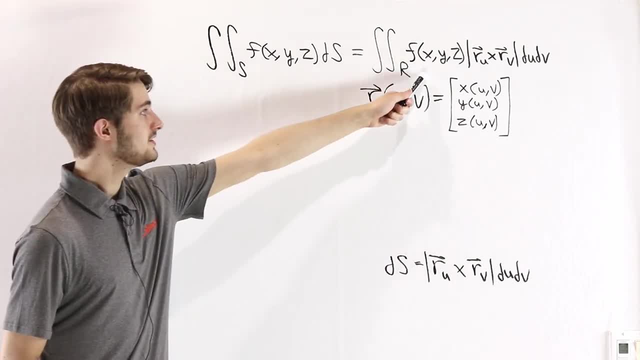 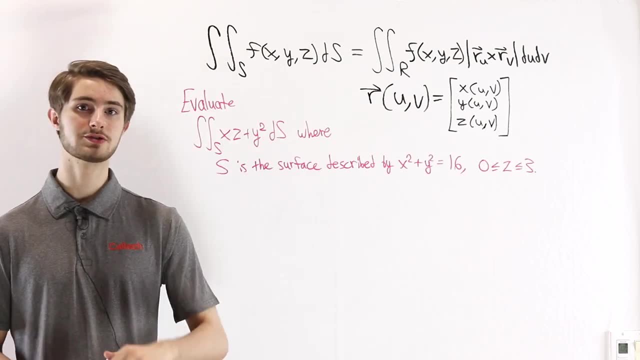 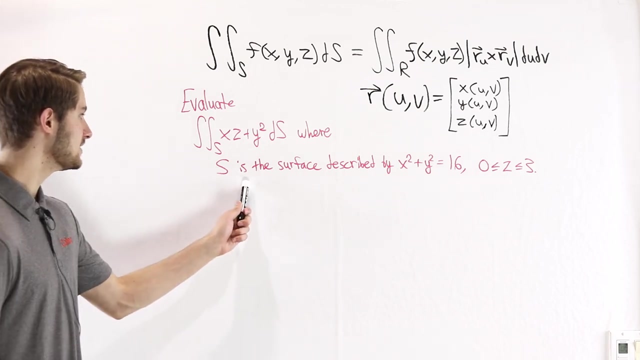 we can easily plug those into the function as well, And so this integral is something that we can actually compute. Now we're going to go through one example of a scalar function. Let's look at a scalar field surface integral. Evaluate the integral over s of xz plus y squared ds, where s is the surface described. 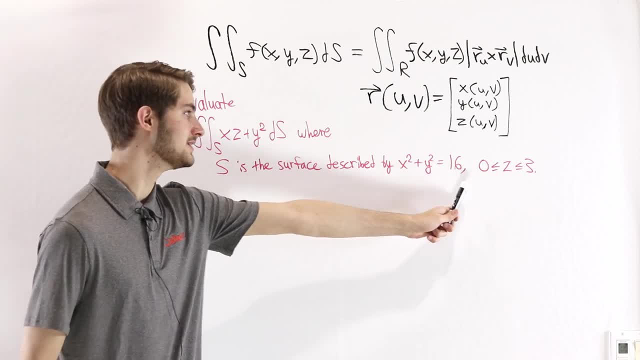 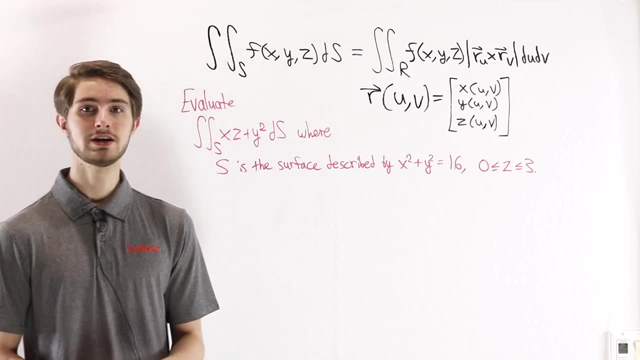 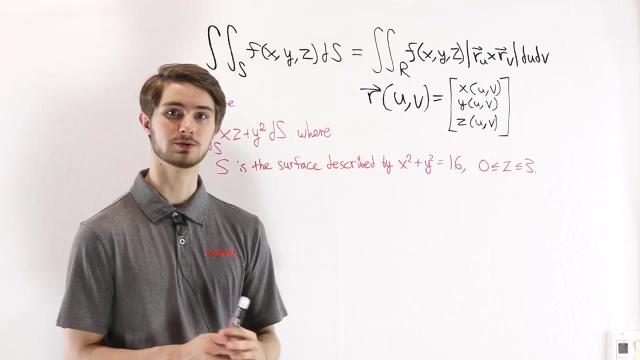 by x squared plus y squared equals 16, for z between 0 and 3.. Just like when we were deriving the formula, the first step here is to get a parametrization of our surface. So let's think about what it means to have x squared plus y squared equals 16.. 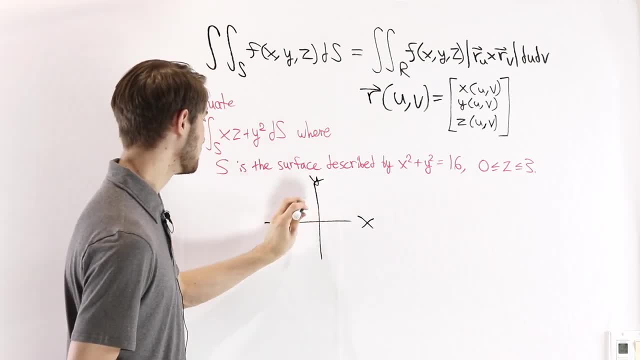 We know that that's going to describe a surface. So let's think about what it means to have x squared plus y squared equals 16.. We know that that's going to describe a surface. We know that that's going to describe a circle in the xy plane where we have a constant. 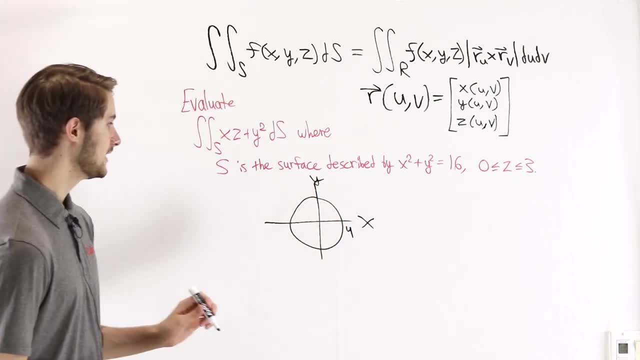 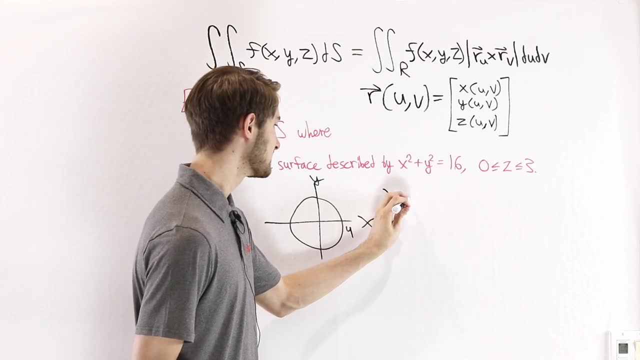 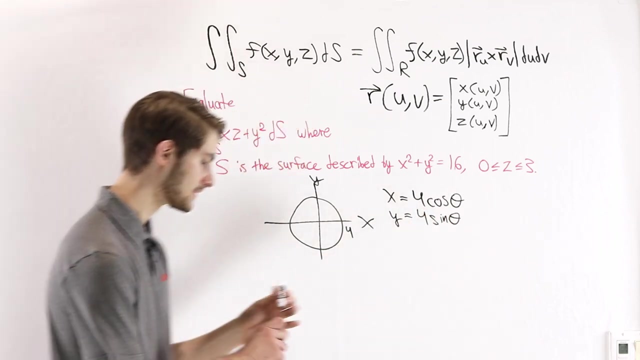 distance from the origin of four. In that case we could use some angle theta to represent every point on the circle. So we would have x equals four cosine theta and y equals four sine theta. So that lets us describe the circle. x squared plus y squared equals 16, but we're not just. 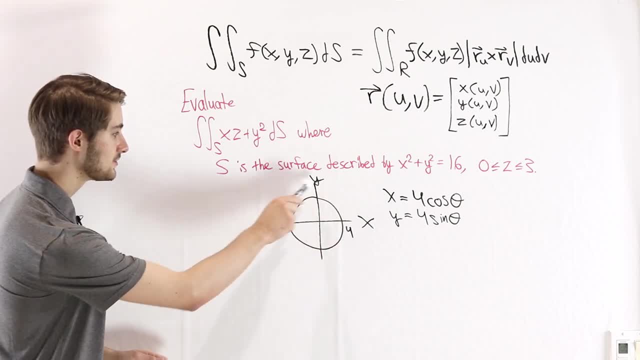 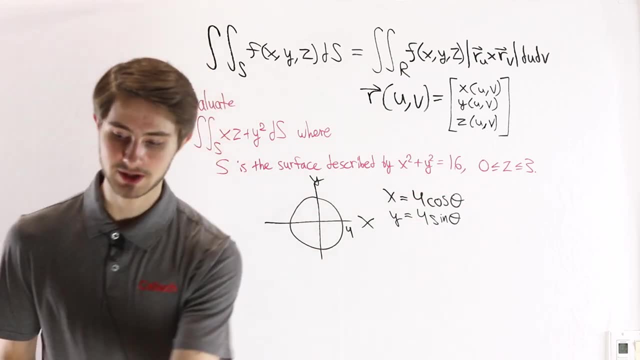 looking at a circle. We're looking at a surface. we take this circle for a range of z values, but notice that this circle stays the same regardless of what z we plug in, and that means that the surface we're looking at is actually going to be. 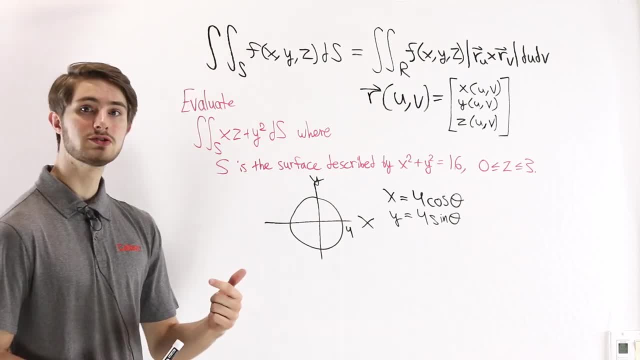 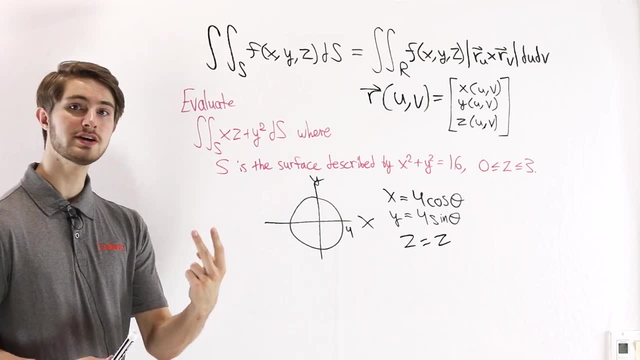 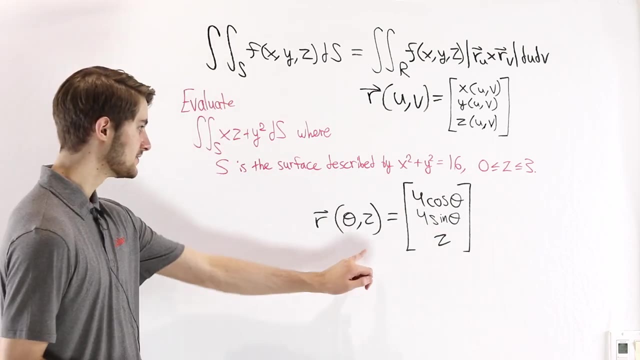 a cylinder. in that case, what we can use as our second variable for the parametrization is simply z. so the two variables that we're going to use to parametrize our surface are theta and z, and we can use the parametrization here. r of theta, z equals our x value, 4 cosin theta. 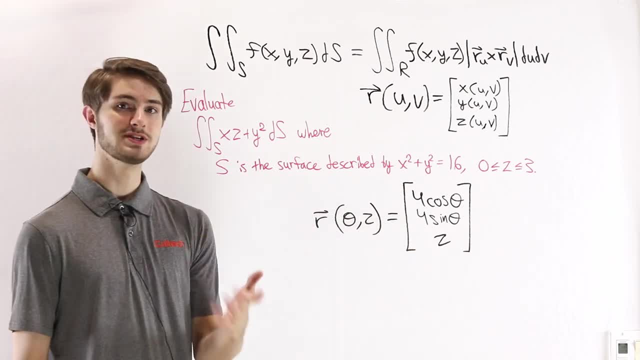 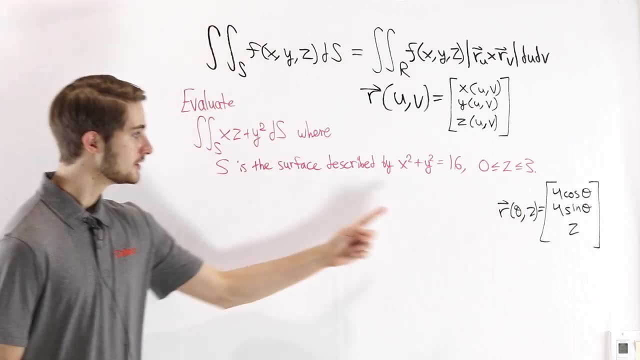 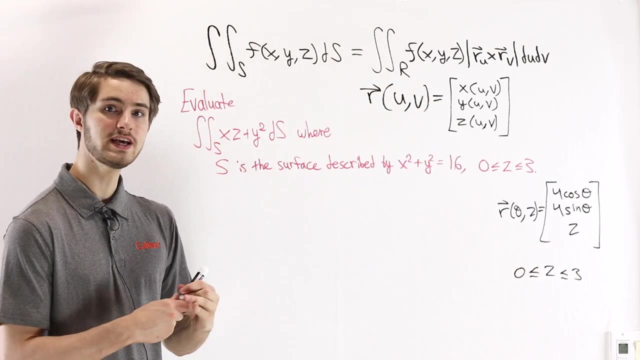 our y value 4 sin theta and our z value just being the variable z. we also need to think about the range of values of theta and z that give us this surface. for the z values, it's pretty clear that we're going to have z between 0 and 3.. For theta, remember that this surface 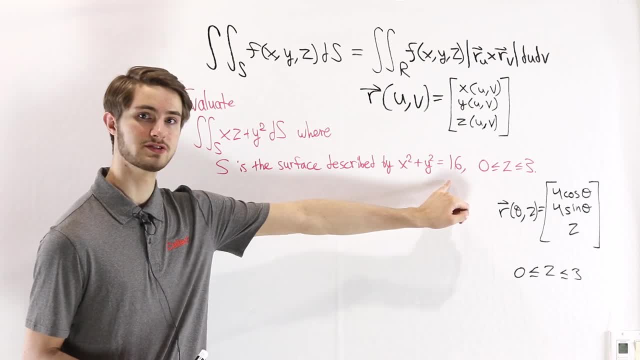 has all of the values, with everything from x to z to theta. give us as sun theta and as r theta, and so on and so forth. squared plus y squared equals 16, meaning we're going to go all the way around the circle. And 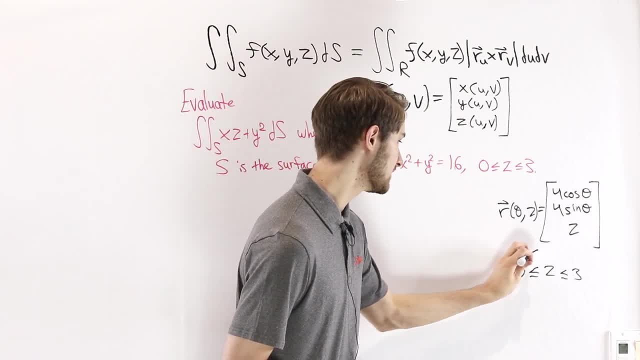 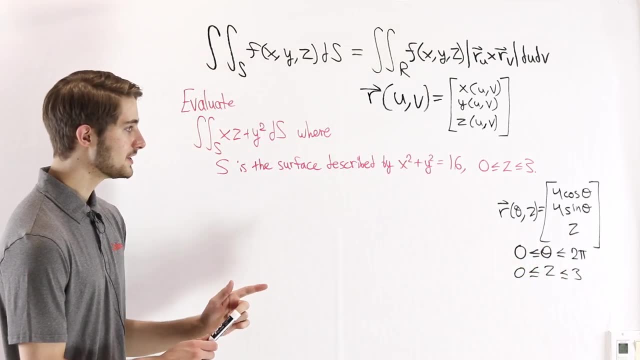 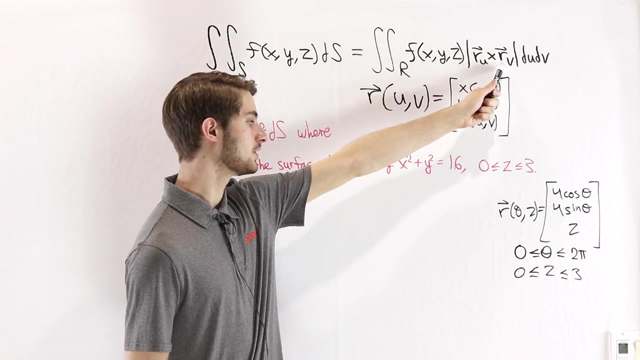 one full revolution of a circle is values of theta between zero and two pi, So that's going to be the range for our theta variable. The last thing that we need to do is calculate the magnitude of this cross product. In our case, that's going to be r sub theta cross r sub z. So we need to figure out. 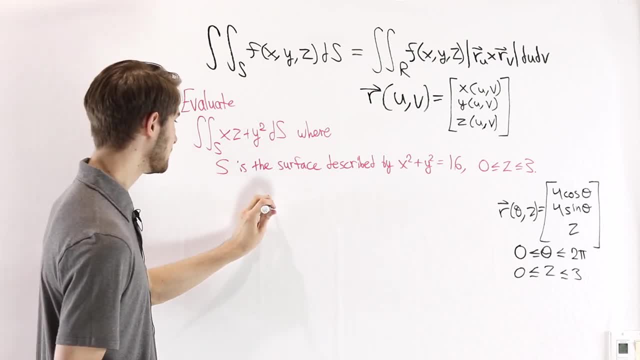 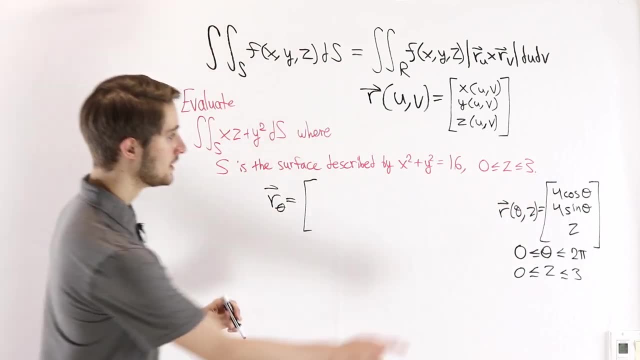 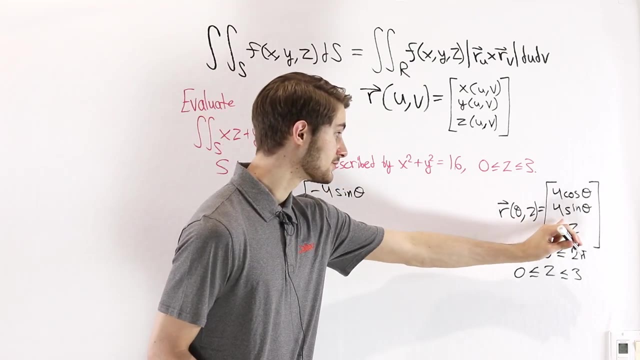 those partial derivatives of this function. First of all, r sub theta. that's going to be the partial derivative of each of these components with respect to theta. For the first one, we're going to have the derivative of 4 cosine theta, which is negative. 4 sine theta, The derivative of 4 sine. 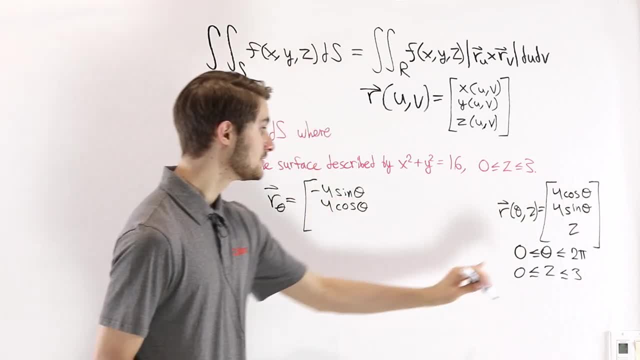 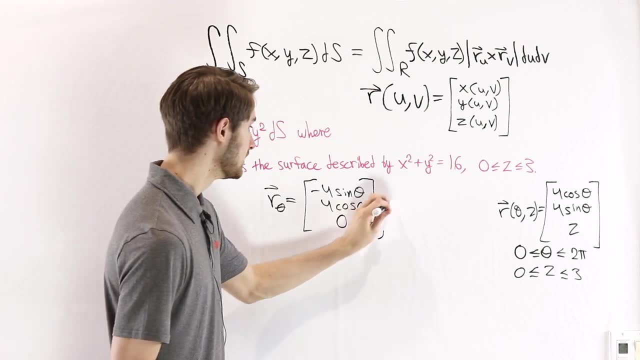 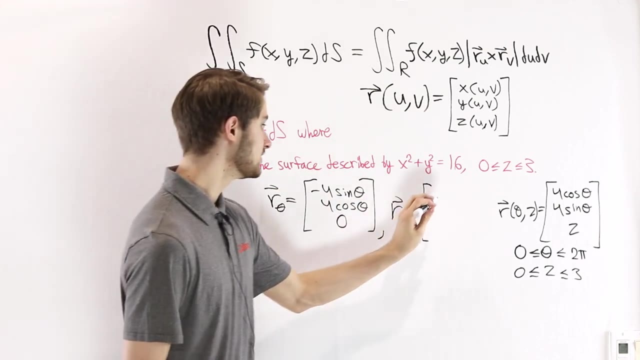 theta will be 4 cosine theta And then the derivative of z with respect to theta is going to be 0, because we're looking at a partial derivative. If we want r sub theta, which we'll sub z, notice that the x and y components are just in terms of theta. so if we differentiate, 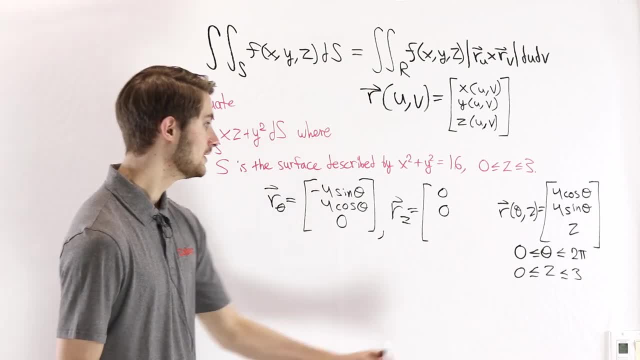 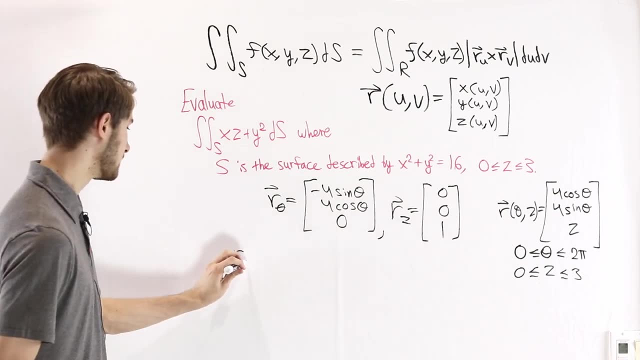 with respect to z, those are constants, the derivative is zero and we have the partial derivative of z, which is just one. Now we need to take the cross product r sub theta, cross r sub z and we can use that determinant. 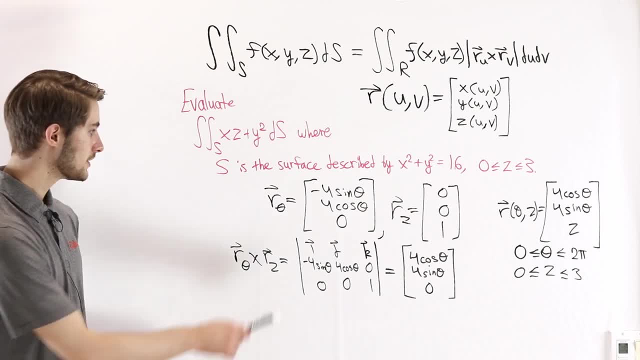 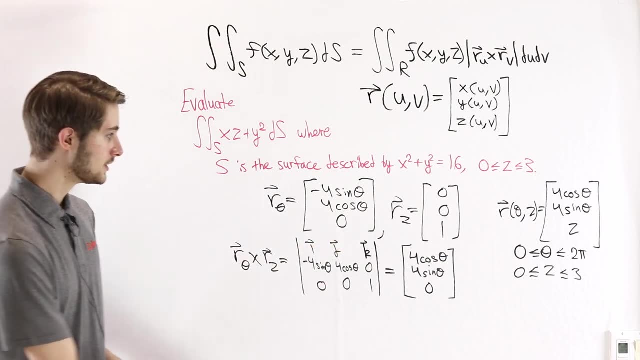 formula to actually compute this. So if we take our two vectors, r sub theta and r sub z, plug them into the cross product formula and compute this determinant, the result that we get is the vector 4 cos theta, 4 sin theta and 0. 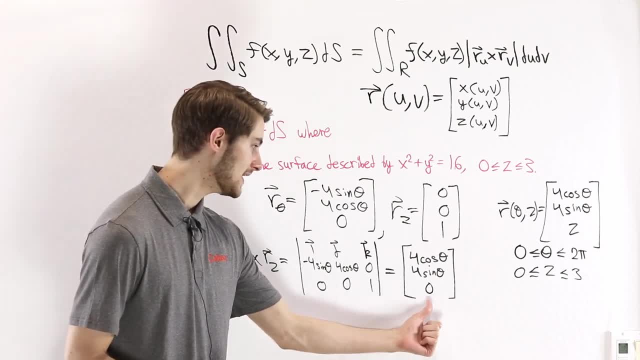 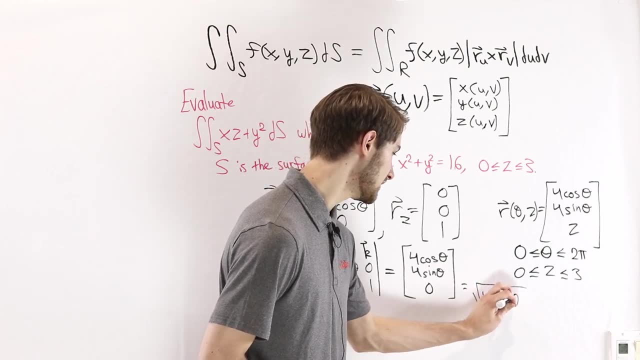 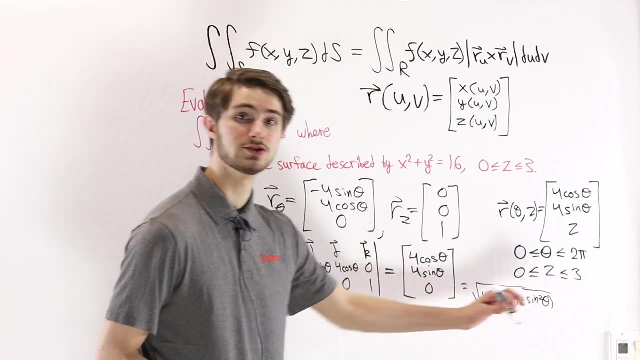 Our goal is to get the magnitude of this vector. So if we take the magnitude here, what we're going to get is the square root of 4 squared times: cos square theta plus sin square theta. And here, cos square theta, theta plus sine squared theta is just 1, so we have the square root of 4 squared, which. 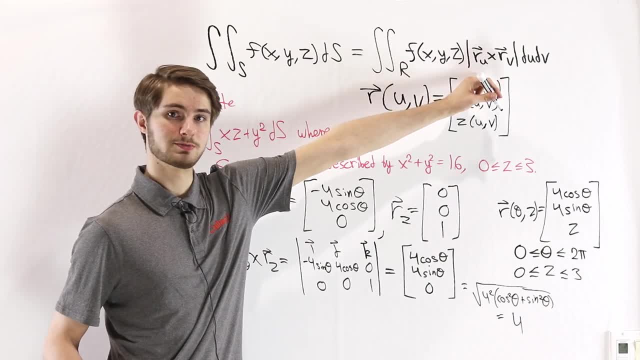 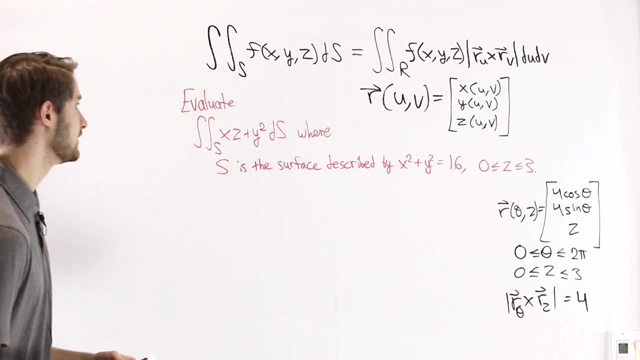 gives us 4.. That's the magnitude of this cross product. Now we're ready to turn this into an actual integral. We can plug everything into the formula that we have right here. First of all, we're going to take the double integral. 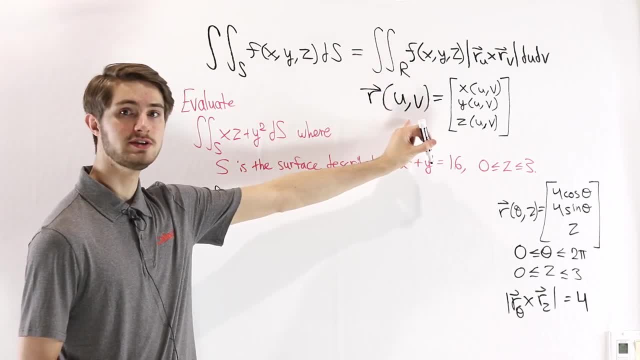 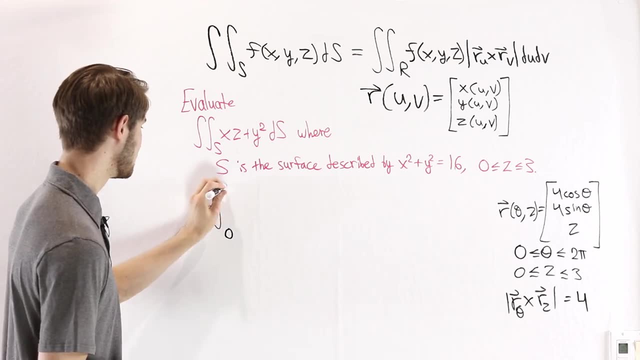 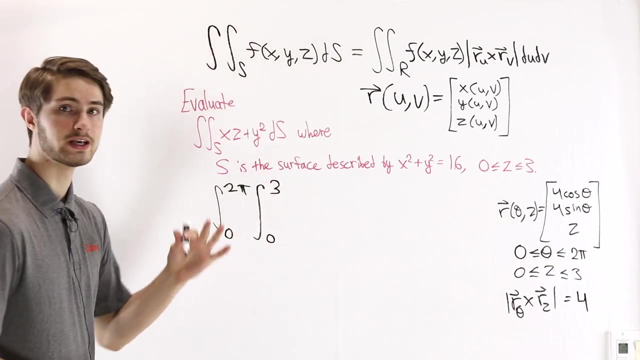 over the region R. that describes the range of u and v values for our surface. We know that theta is going to go between 0 and 2 pi on our surface and we know that z is going to go between 0 and 3.. So that gives us the range for our double integral. Then we want: 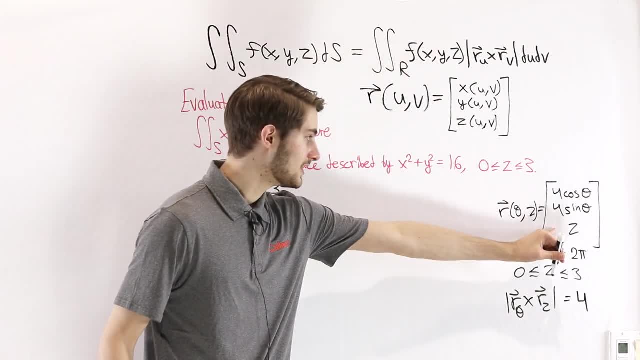 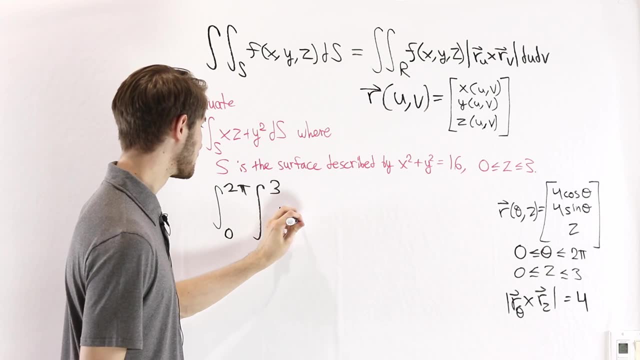 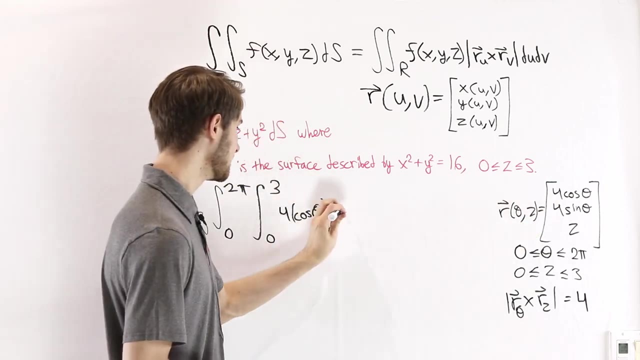 f. We know that x, y, z values are described by this vector over here. so if we want x times z, that's going to be 4 cosine theta times z, and then we add y squared, which is 4 sine theta squared. From here we're going to multiply this entire expression. 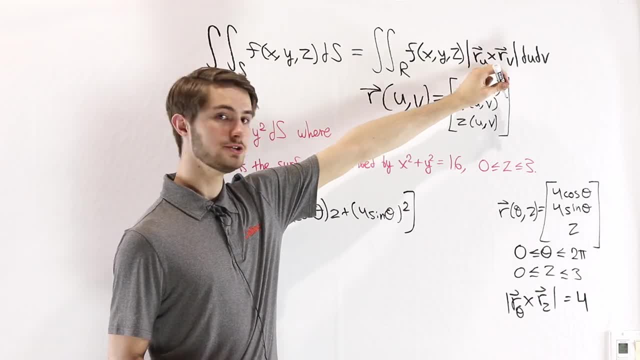 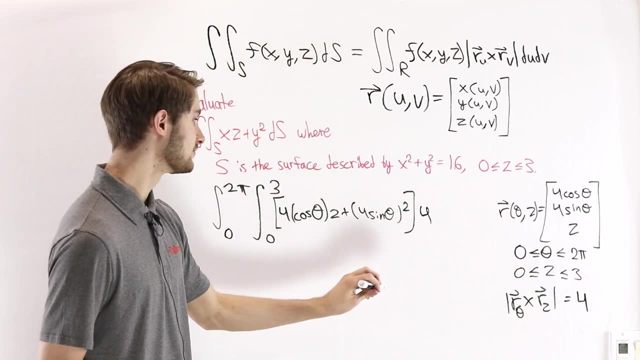 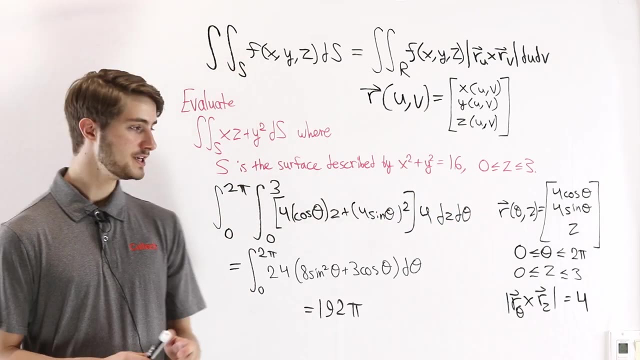 which is just f times the magnitude of our cross product. We got that the magnitude of the cross product was equal to 4, so we're just going to multiply a 4 out here. dzd, theta. Since we're focusing on surface integrals in this video, I'm not going to go through. 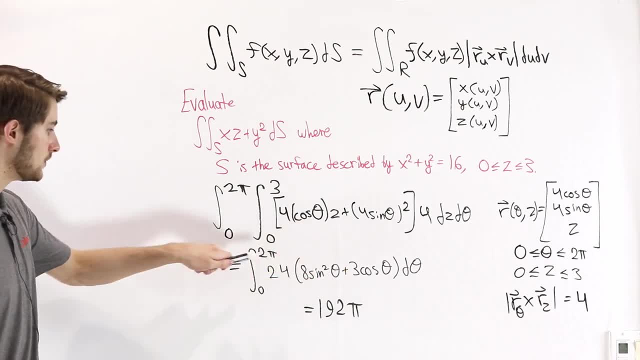 all the computations of this double integral, but I'm going to show you how to do that. So we're going to go ahead, and we're going to go ahead, and I've written out one step in the process here and I've written our final. 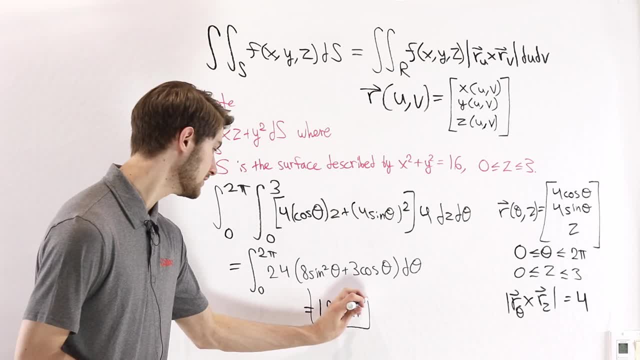 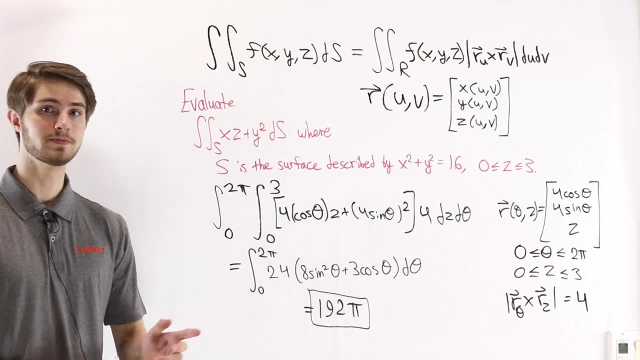 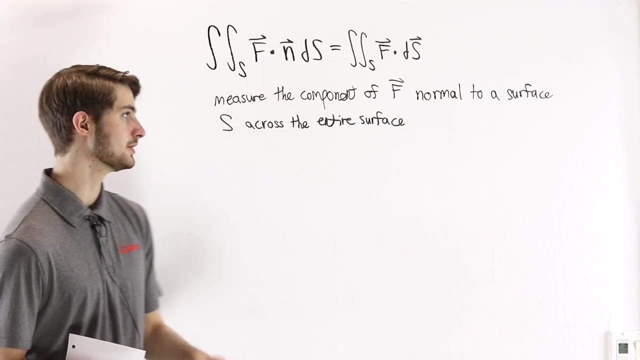 answer if we evaluate this integral, which is 192 times pi. So that's all we need to do to evaluate a surface integral in a scalar field. And now it's time to start looking at vector fields. So the purpose of a vector field surface integral is to measure the component. 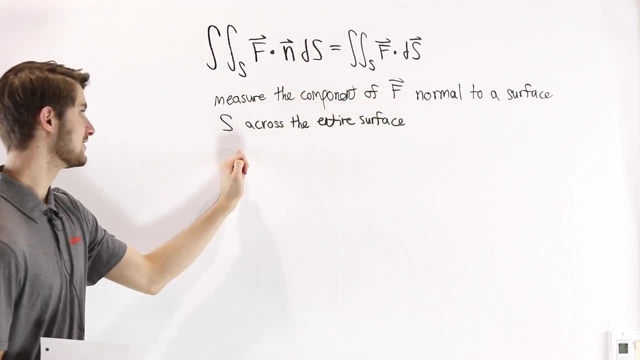 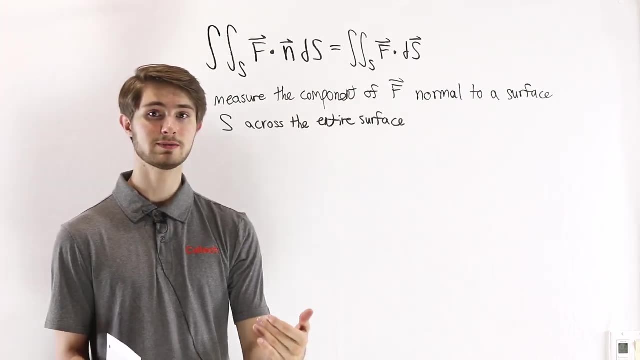 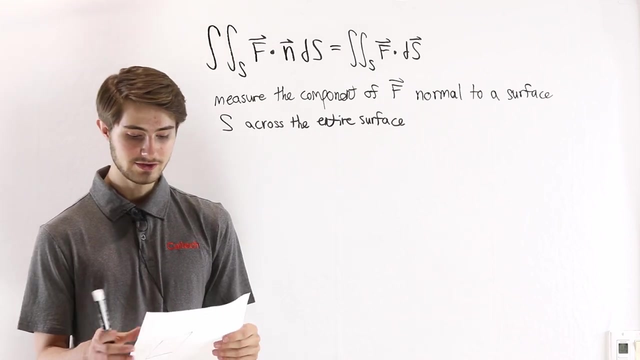 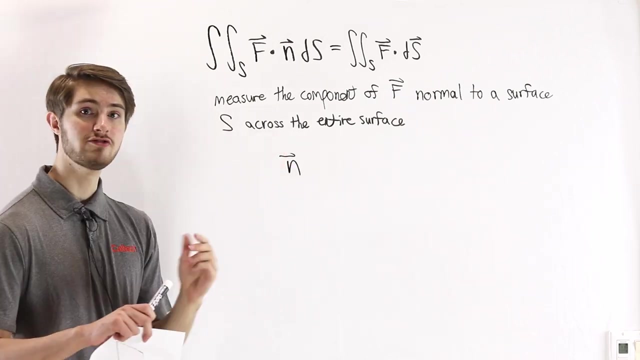 of some vector field f normal to a surface s across the entire surface. In order to do that, we can think about taking our surface and constructing a unit normal vector, A vector that by definition, is normal to the surface, pointing straight out of the surface at a. 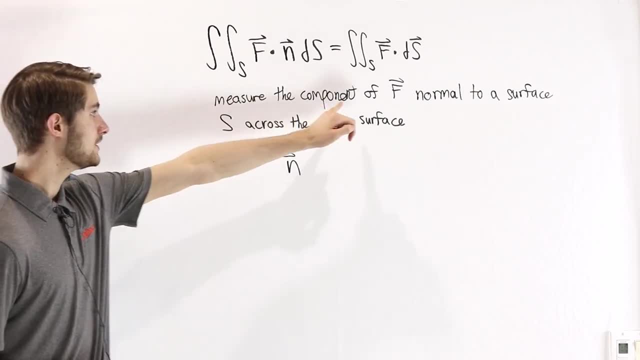 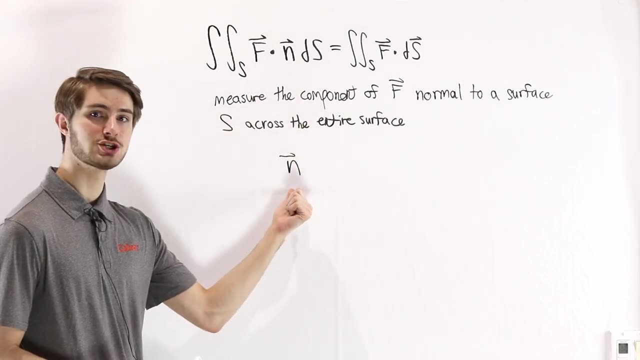 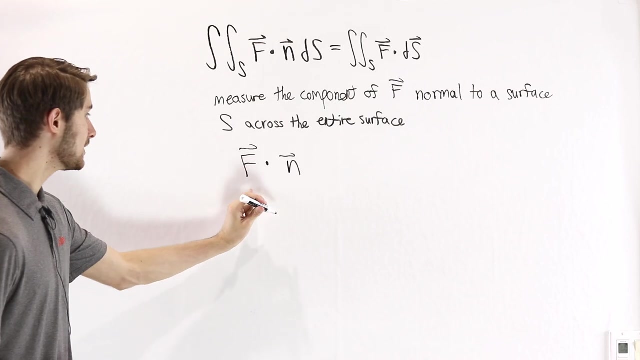 particular point. Now, if we want to measure the component of f normal to the surface, that's the same thing as measuring the component of f in the direction of the normal vector. And the way that we do that is with a dot product. If we take the dot product of f with 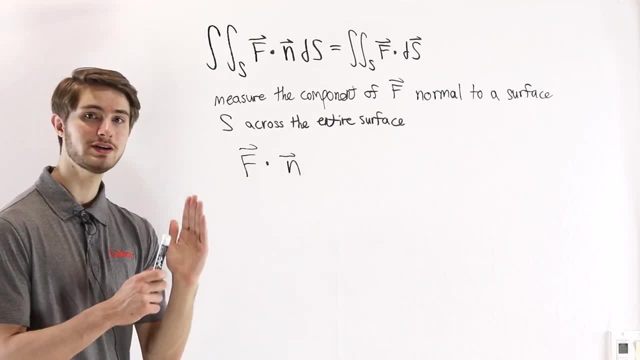 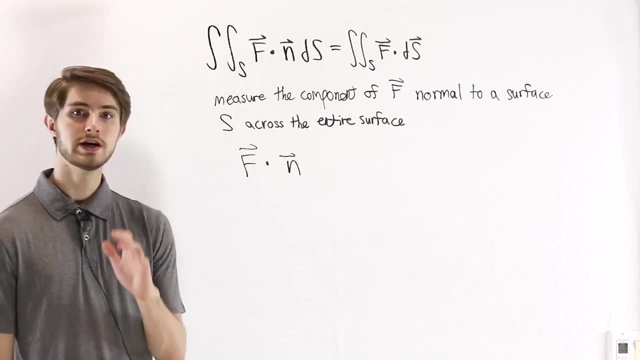 a unit normal vector n that gives the component of f in the direction of n, because the dot product talks about how parallel the two vectors are. Now remember that f, dot, n is a numerical value, it's just a number that represents the component. 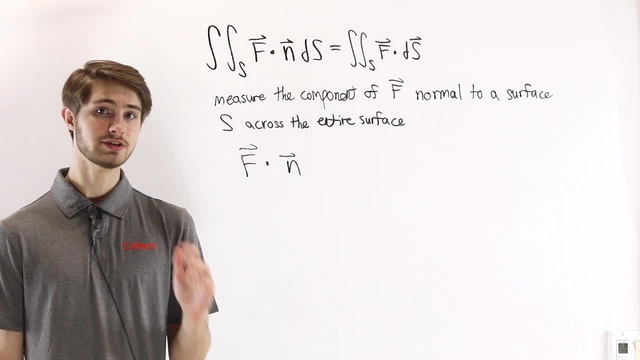 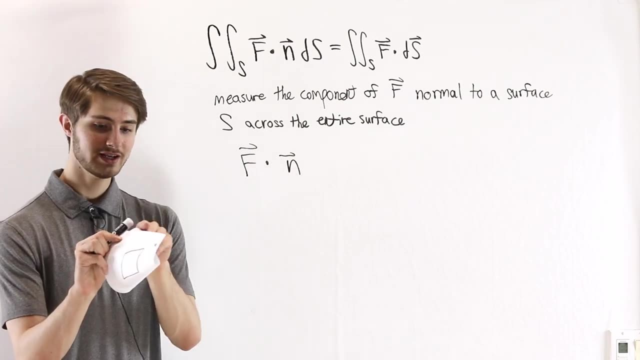 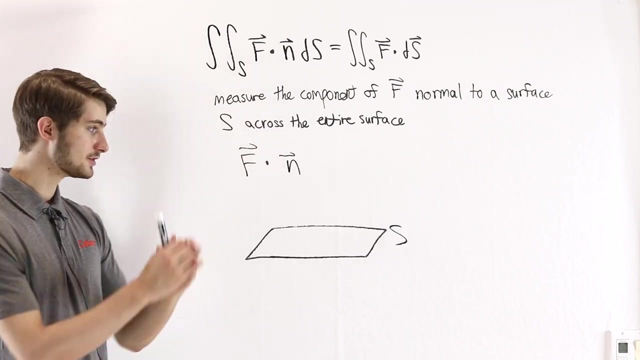 of f in the direction of n And because it's just a number, we can make a graph of it. In order to graph f dot n, we'll start by taking our surface s, and flattening it so that it becomes a two dimensional region. So let's say we flattened our original surface. 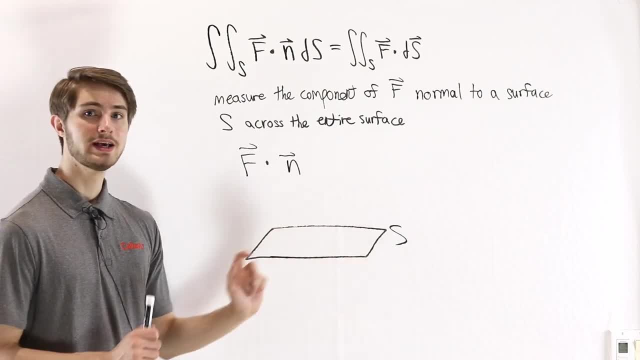 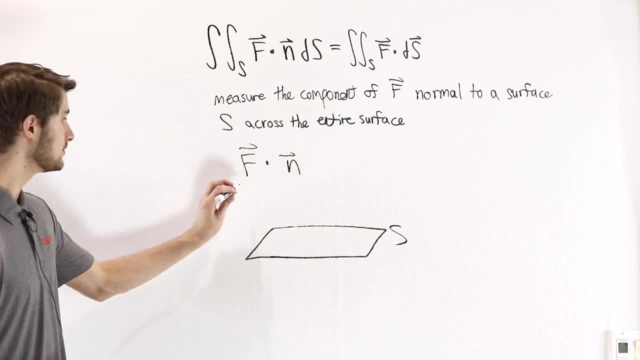 s and got this two dimensional region right here. In that case we can take f dot n for every point along this surface and that's going to correspond to the point where the acted out storage is located, or at every point in our surface. 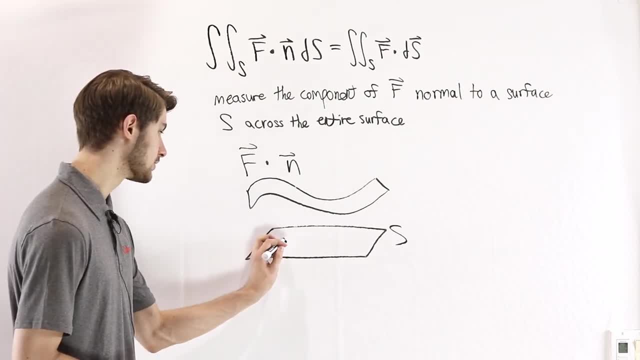 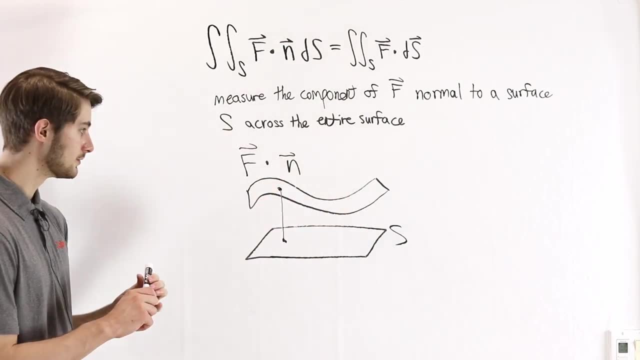 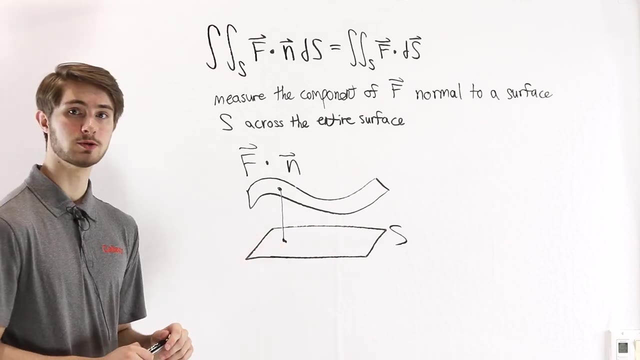 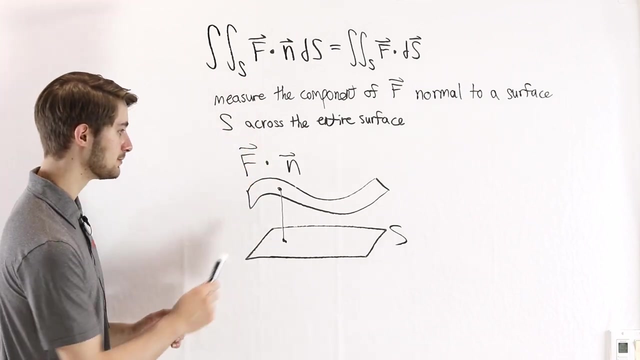 At every point on this two dimensional region here corresponding to some point on the original surface S, the height above that point represents f dot n. at that point, If, instead of considering just a single point, we want to aggregate all of that information and look at the entire surface instead of just taking the height at a point, we'll just 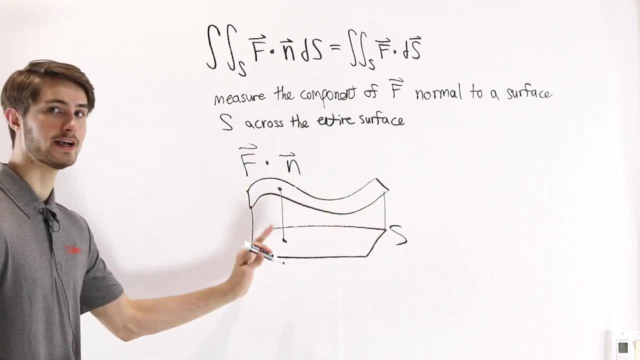 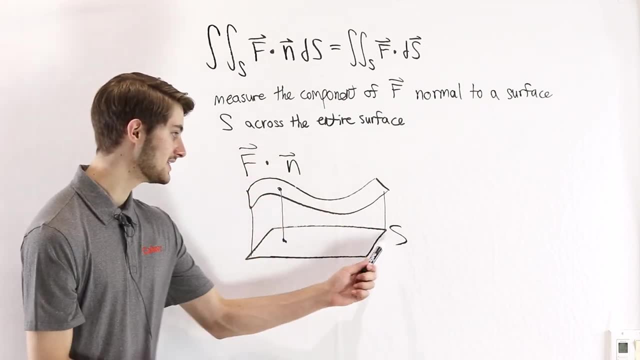 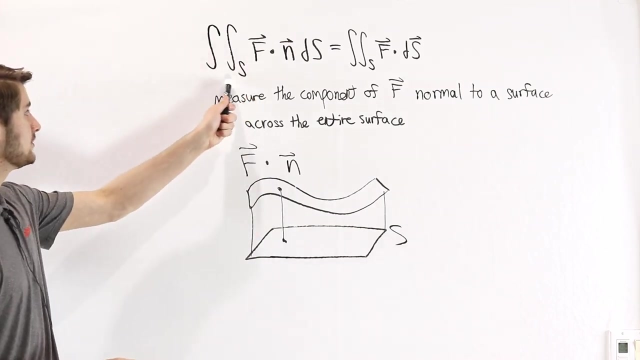 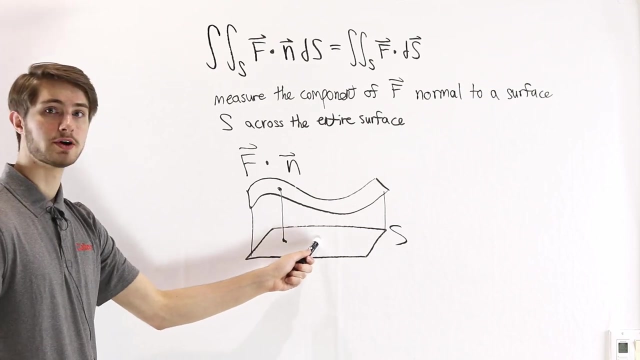 we can take the volume under the entire shape And the volume of this function, fn, above the two-dimensional region representing s. that is what we call the vector field surface integral, which we denote by the integral over our surface s of fn times ds, where ds is the area of a small 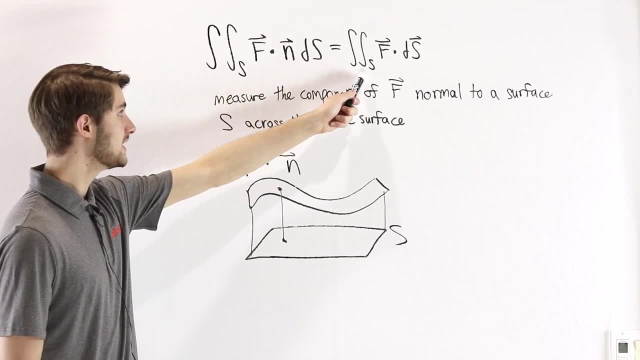 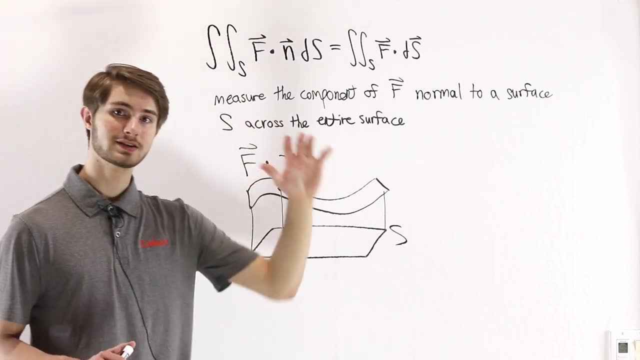 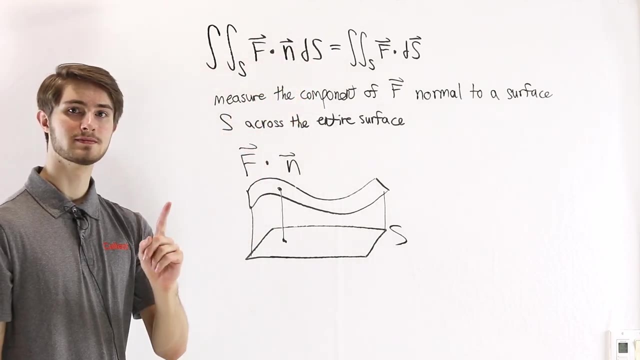 part of that original surface. We also sometimes write it as fds, where ds is itself a vector, and that's because once we get to the computation it's often easier to group n? ds together as just one thing. From here, turning this vector field surface integral into something we can actually 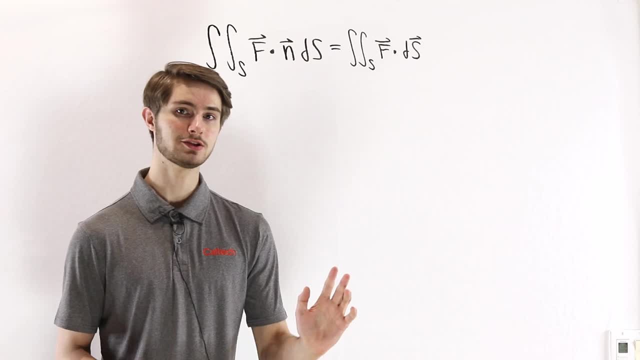 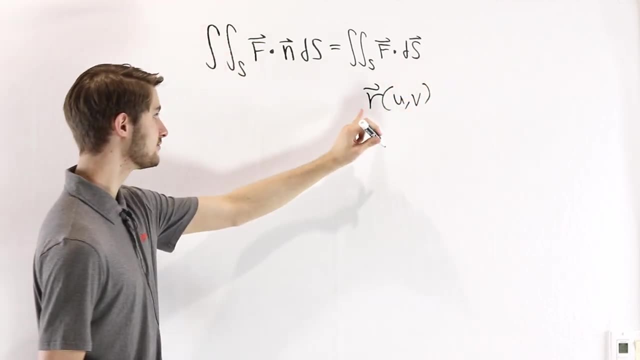 compute follows a lot of the same steps as we did with scalar field surface integrals. Just like before, our first step will be to change the vector field surface integral into something we can actually compute. We can parametrize the surface in terms of some function r of u and v. 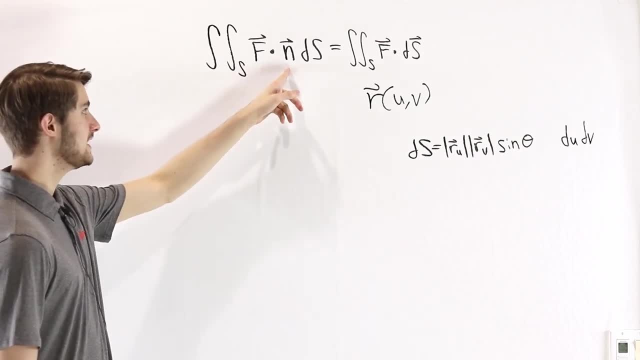 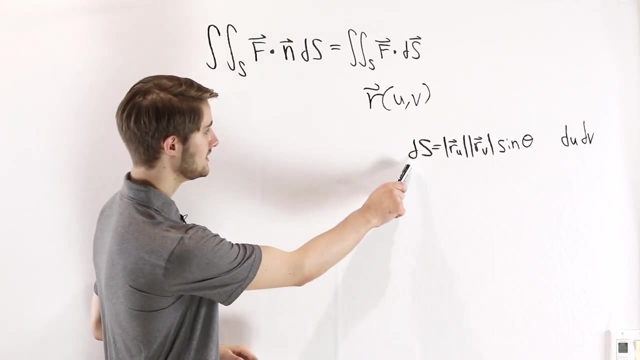 Then we need to figure out how to find the unit in normal vector n times ds. We can start with the formula that we found when we were doing scalar field surface integrals: that ds is equal to the magnitude of r sub u times the magnitude of r sub v times the sine. 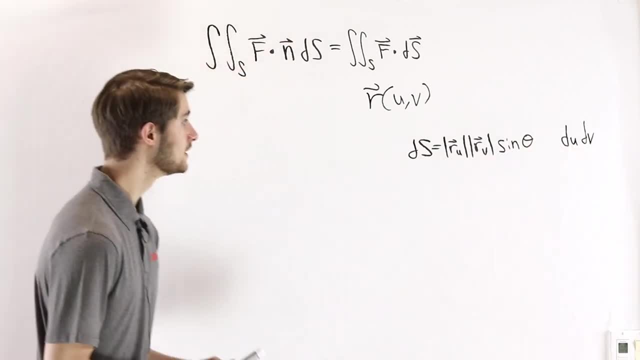 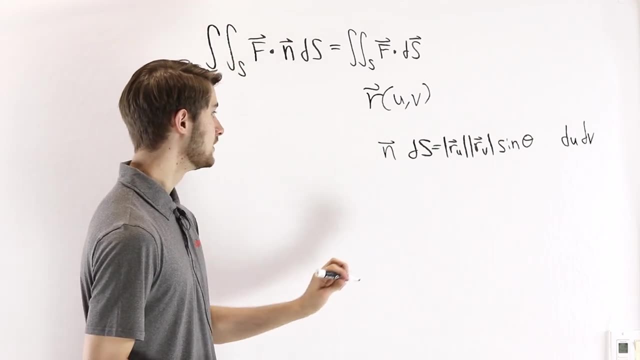 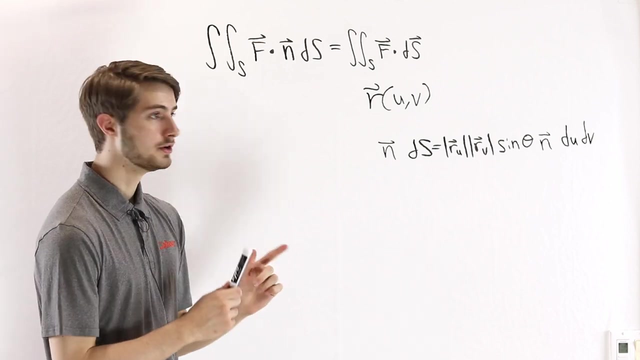 of the angle between them. times du, dv. From here we don't just want ds, we want n ds. But if we want the unit normal vector on the left side, we can also multiply it on the right side over here- Notice what this part of the formula is- We have the magnitude of the first. 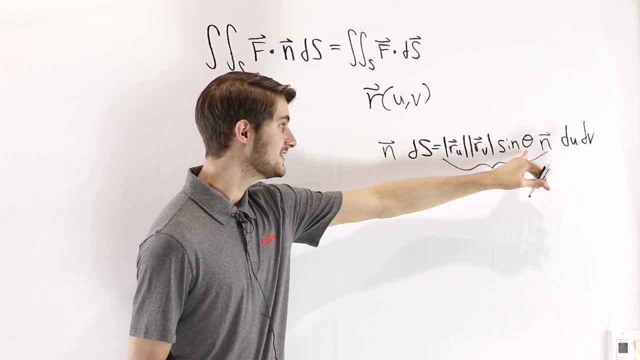 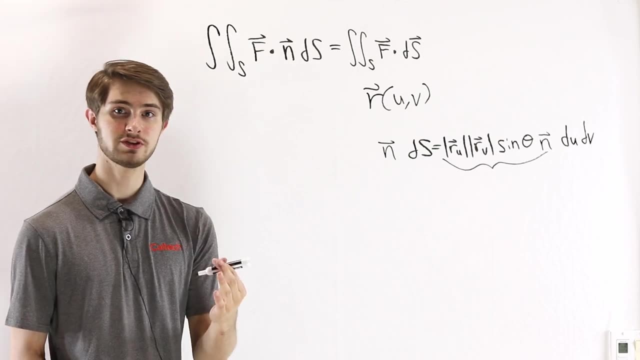 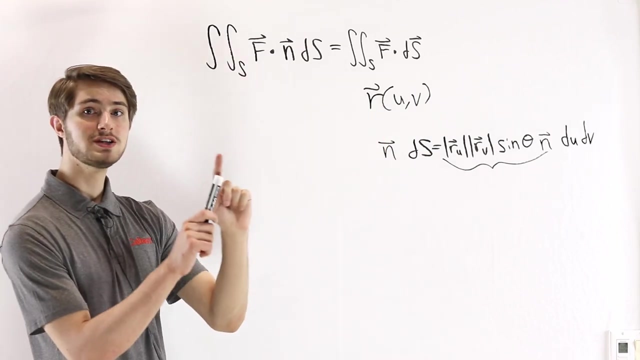 vector times the magnitude of the second vector, times sine theta, times a unit normal vector. This unit normal vector is normal to the surface, but remember that r sub u and r sub v are partial derivatives of our vector function, which means they are going to move along the surface. 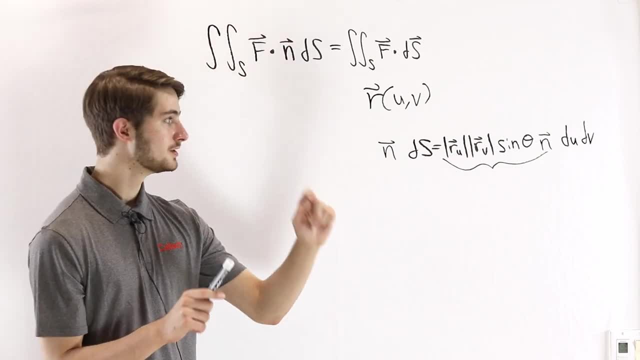 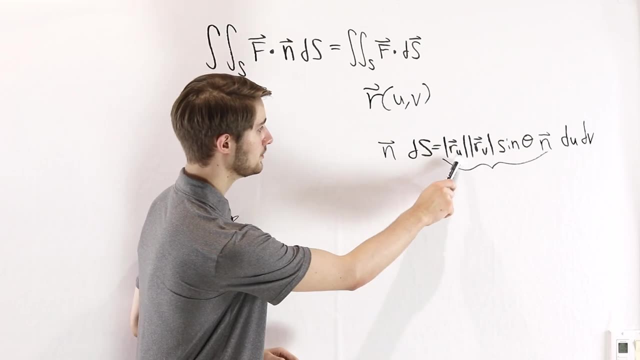 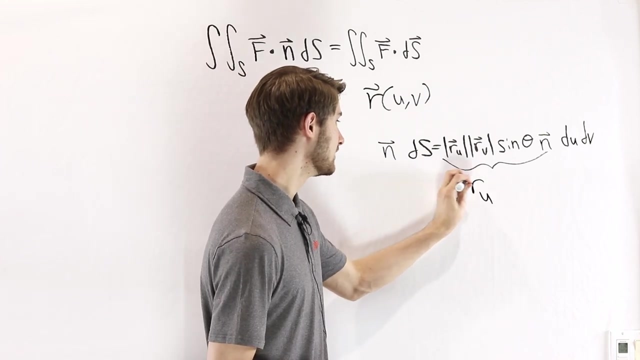 Both of these vectors represent movement in the surface. So this unit normal vector here, because it's normal to the surface, it's also going to be normal to both of these vectors And therefore this entire formula here is the exact formula for r, sub, u cross, r sub. 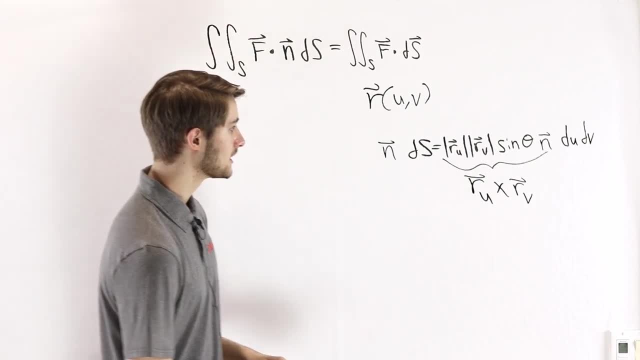 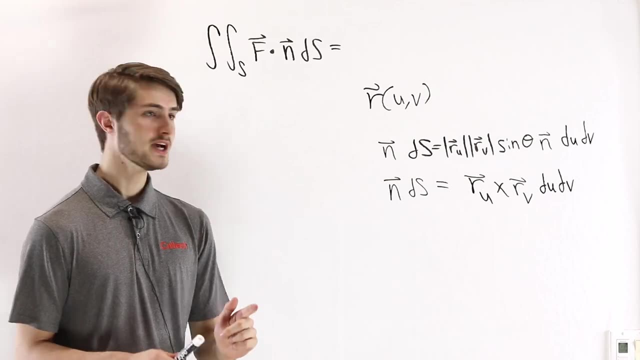 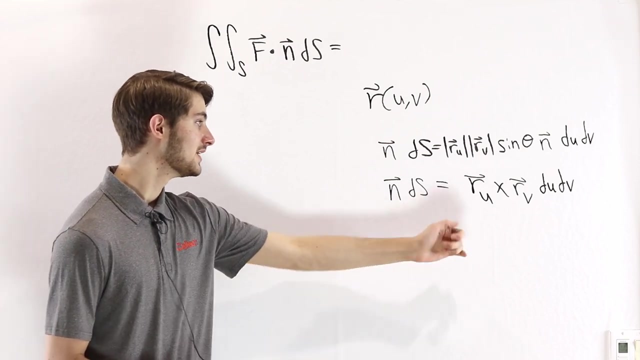 v. We don't even need the magnitude this time, because this unit normal vector represents the direction of that cross product. So when we have a parametrization r of uv that describes our surface, we can write the unit normal vector times ds as r sub u, cross, r sub v, du, dv. 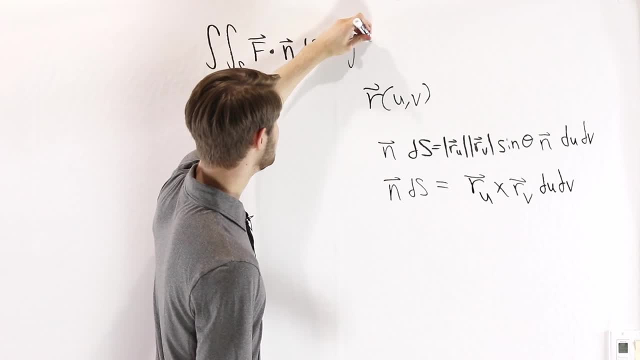 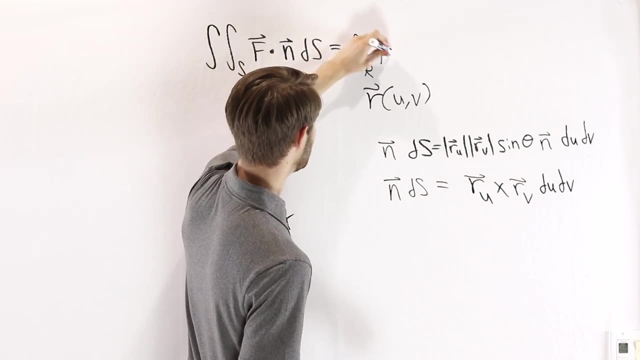 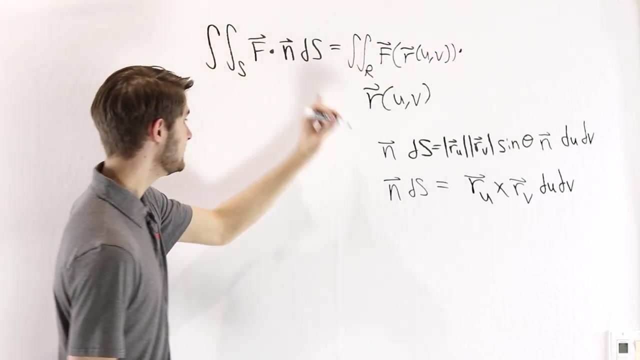 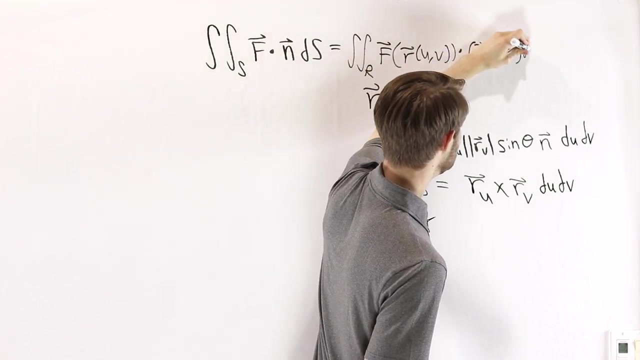 And therefore we can turn our original surface integral into a double integral over a region r of uv values. that gives our surface Of the vector field f evaluated at the point on the surface r of uv, dotted with n? ds, which is what we have right here: r sub u cross, r sub v du dv. 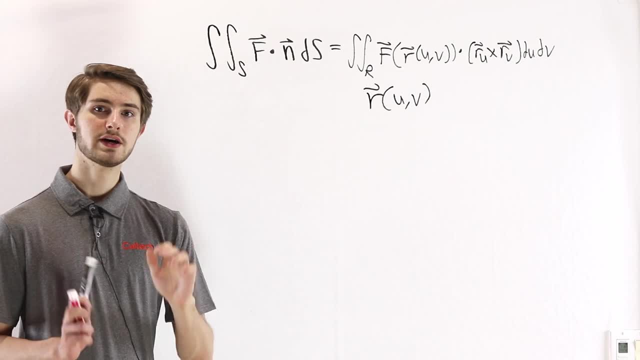 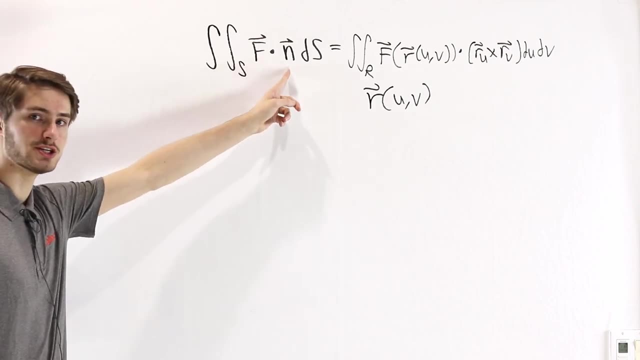 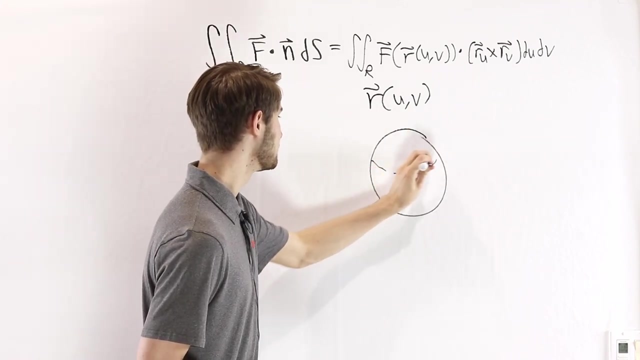 And that's all we need to compute the surface integral. Now there's one more thing that we need to understand with vector field surface integrals, and that is to pay attention to the orientation of the unit normal vector To see what that means. let's say, the surface that we are looking at for our integral is: 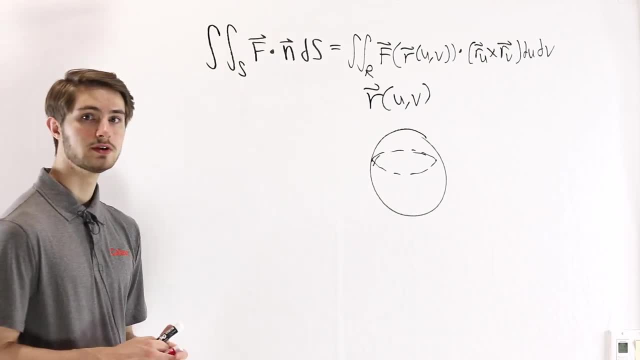 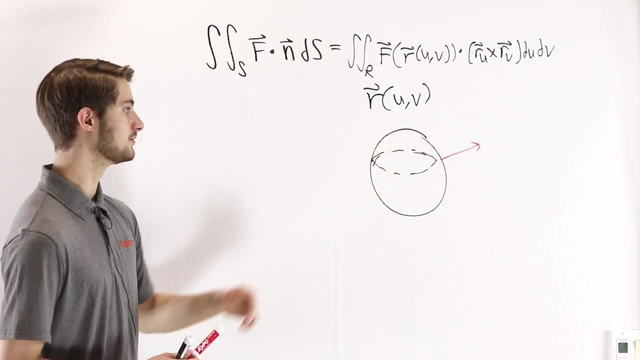 the surface of a sphere. In that case, we could have a unit normal vector that points off of the sphere, just like this. That would be normal to the sphere. However, there is another unit normal vector that we could have chosen instead. 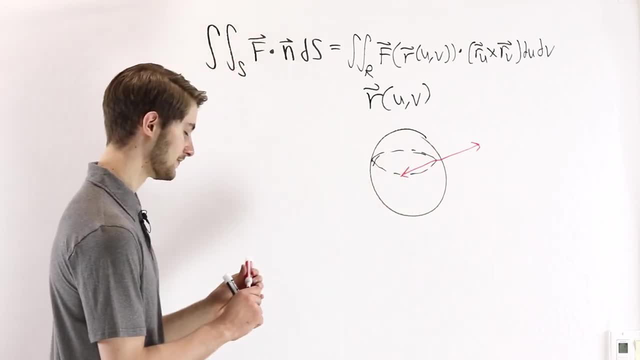 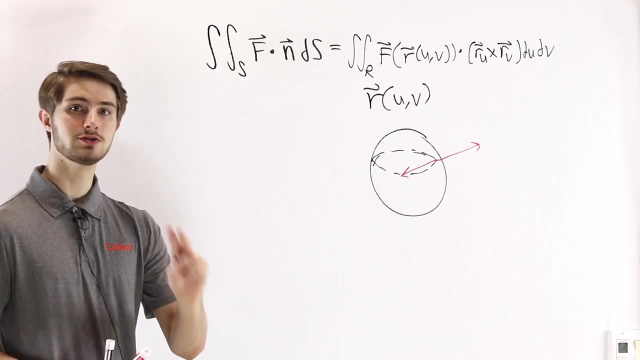 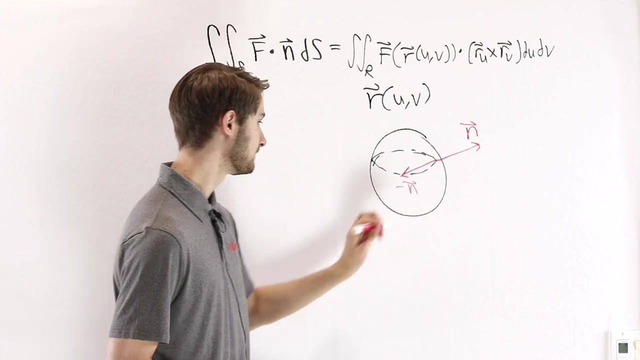 And that is the unit normal vector that looks like this, The vector pointing in the exact opposite direction direction. So there are always two unit normal vectors to a surface. There is the original vector n and there is negative n When we do a vector field surface. 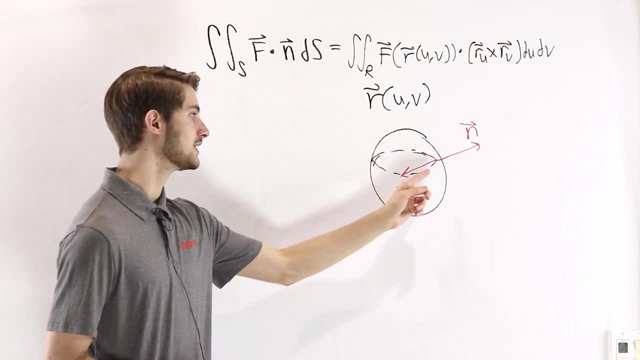 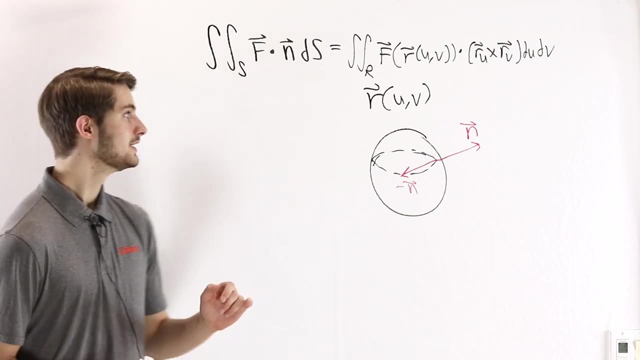 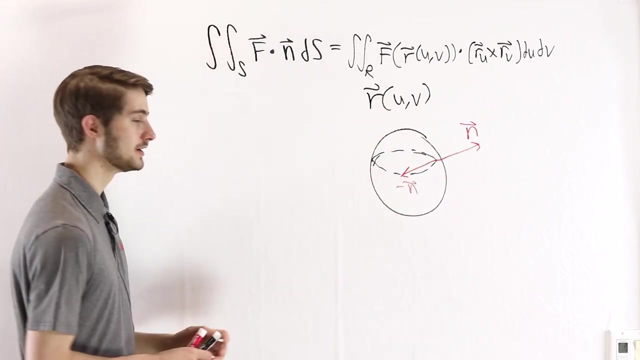 integral. we always have to recognize that we're choosing an orientation for the normal vector. Now, when problems describe the normal vector, they'll usually say that it's either upward versus downward or outward versus inward. In the case of the sphere here it would make sense to describe the normal vector. 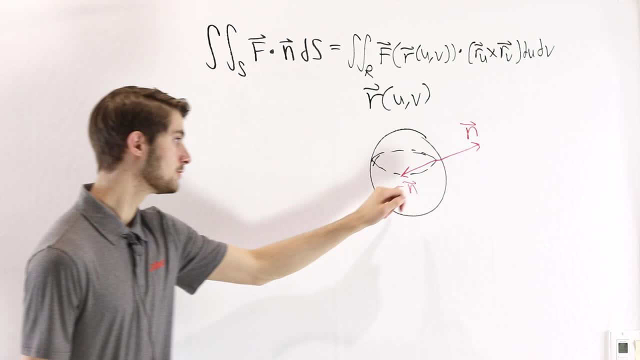 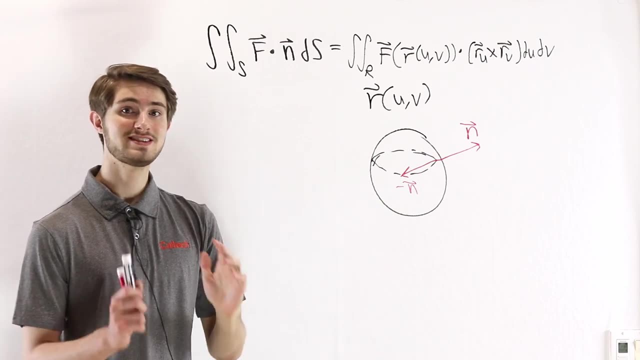 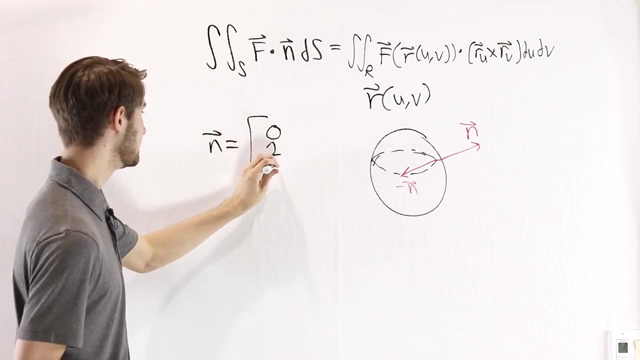 as either pointing outward, away from the sphere, or inward, towards the center of the sphere. When the normal vector is described as upward versus downward, that's talking about the z-component of the normal vector. So if our normal vector, for example, were 0,, 2, negative, 1, we could tell that this normal vector 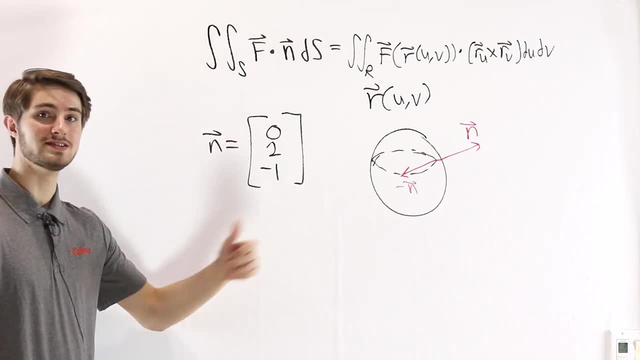 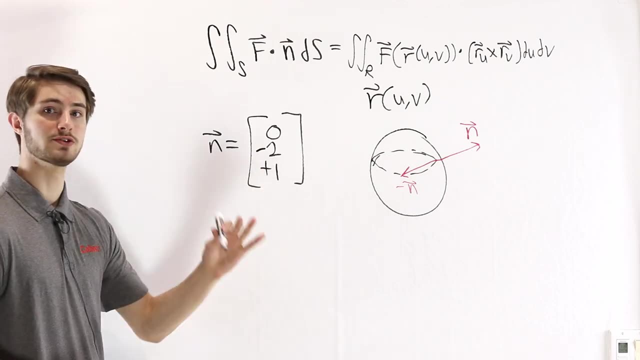 would be oriented downward because the z-component is negative. If we were to do a vector field surface integral, we would have to find the z-component of the normal vector. If we wanted it to be oriented upward, we would take the negative of this vector so that the z-component was positive. Now, when the 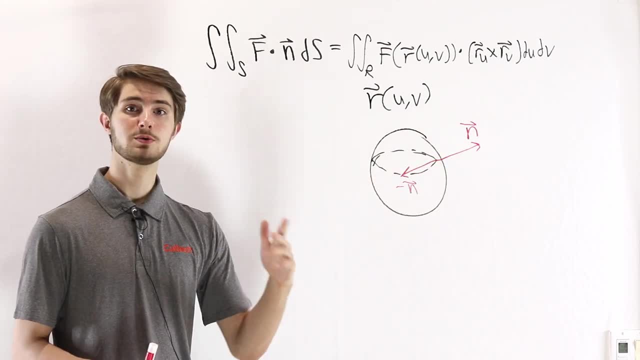 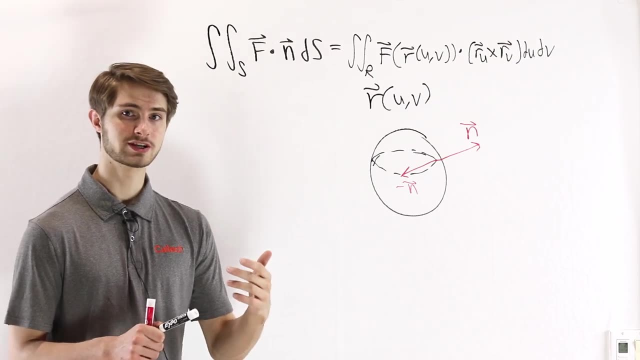 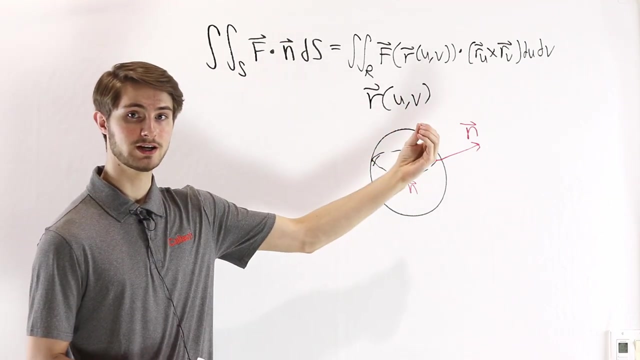 normal vector is described as inward versus outward, it's not always as clear which direction our normal vector is pointing. So in those cases, if we can't tell whether our normal vector is pointing in the right direction, what we can do is choose some values for u and v, just plug in some values there: determine: 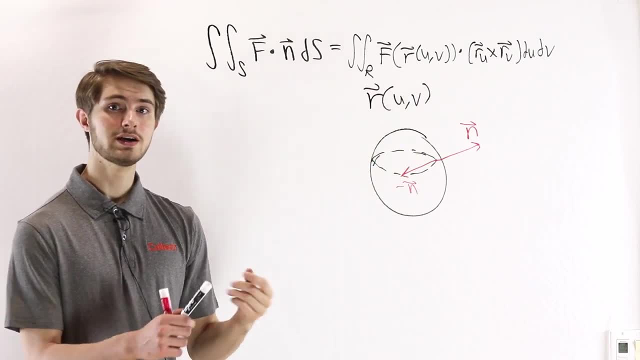 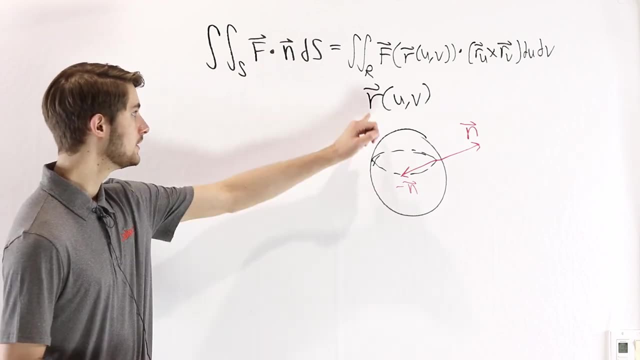 the point on the surface and the normal vector. If we want the point on the surface to be pointing in the right direction, we can plug in some values there. For example, let's say that our surface is this sphere. here, If we took our parametrization and plugged in a certain value for u and v, we would get a specific. 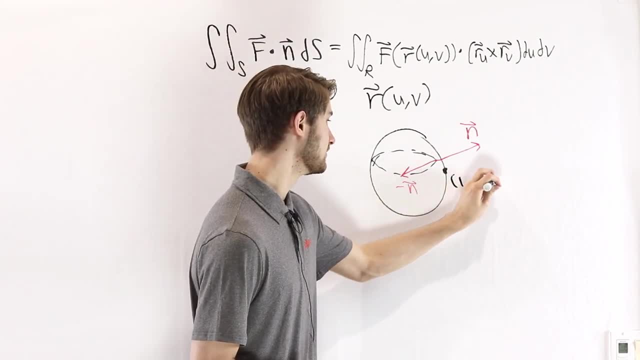 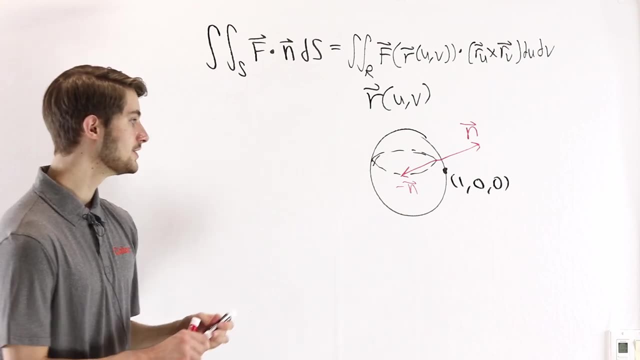 point on the sphere which say is 1, 0, 0. Then we can plug in those same values for u and v to get our unit normal vector And say that our unit normal vector at this point was equal to negative 1, 0.. 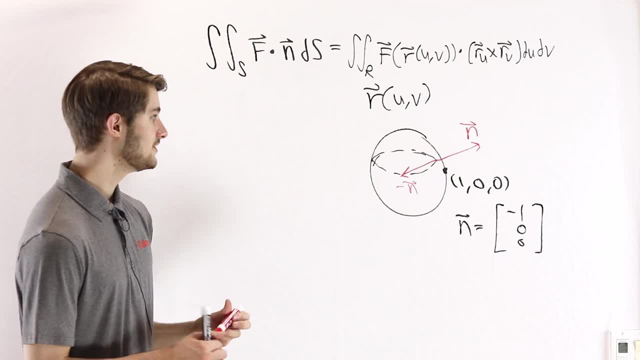 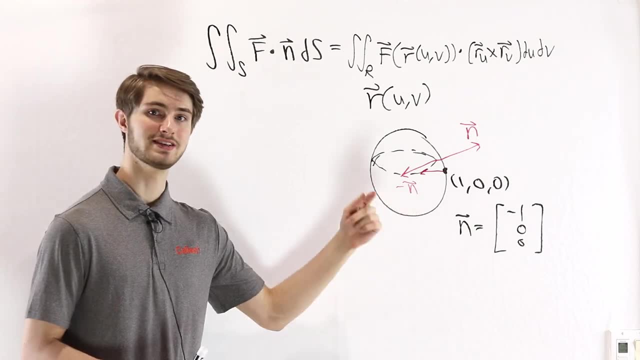 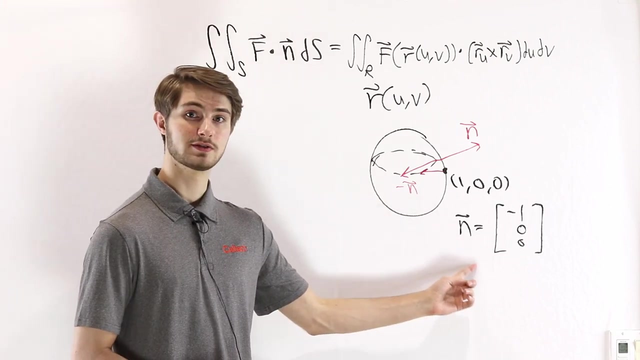 From there it's pretty easy to see that our normal vector is going to point back towards the center of the sphere and therefore it is oriented inward From there. if the problem said the normal vector is oriented outward, we would need to take the negative of our normal vector so that we got the proper orientation. So 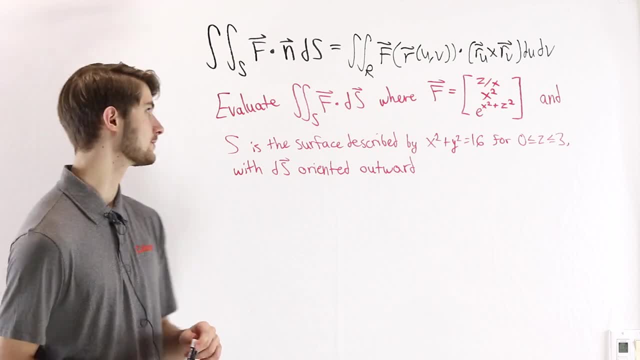 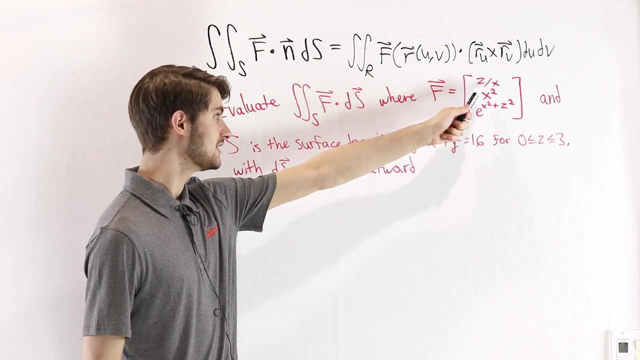 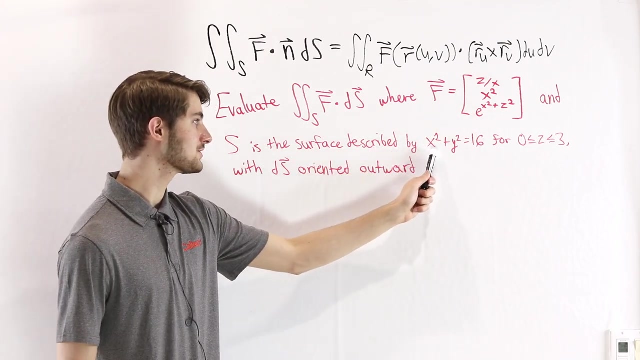 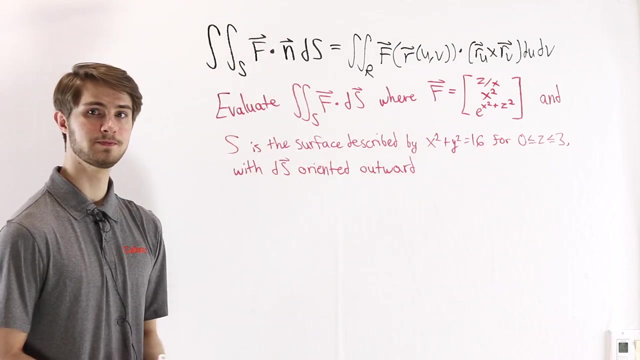 now we'll go through an example of a vector field surface integral. Evaluate the integral over s of f, dot ds, where f is z over x, x squared, e to the x squared plus z squared and s is the surface described by x squared plus y squared equals 16 for z between 0 and 3, with ds oriented outward. 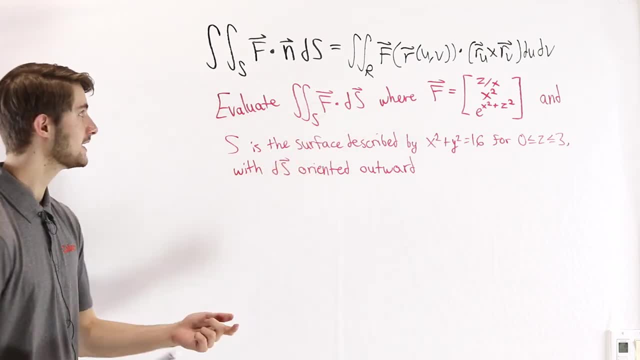 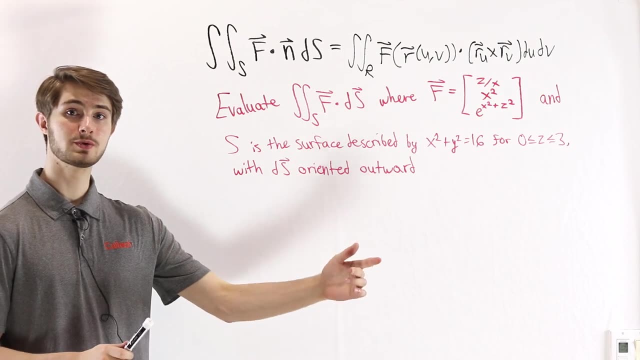 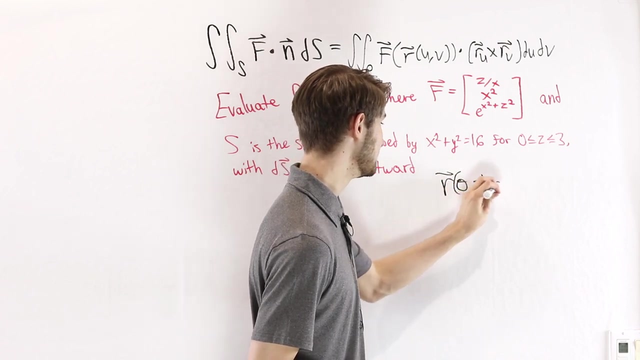 Remember that in this case, ds- this vector is just a shorthand for the unit normal vector times ds. In this case, the surface s is the exact same surface as we were looking at with the scalar field surface integral, Which means we can use the same parameterization- r of theta and z as 4 cosine, theta, 4 sine. 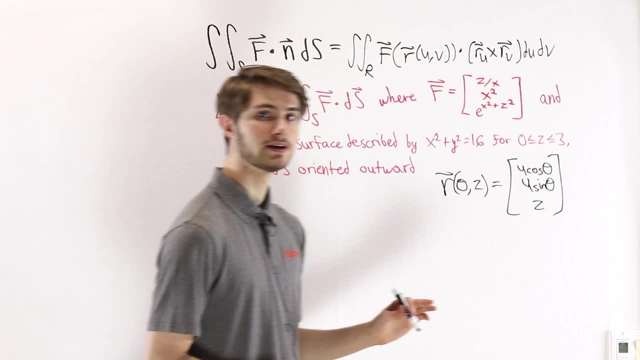 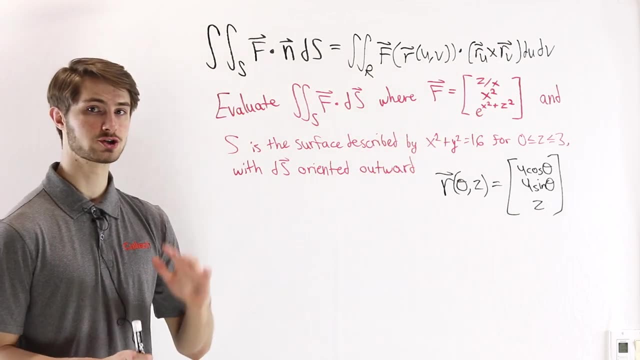 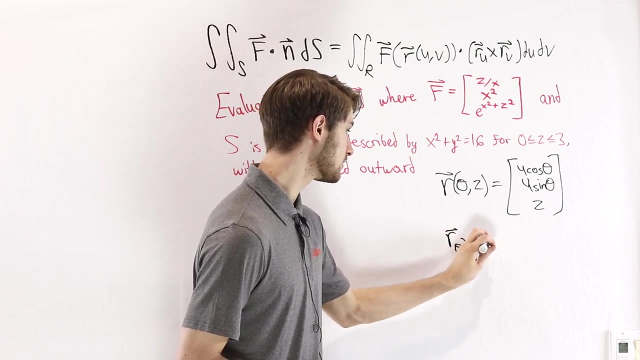 theta and z And from there we can also use the same cross product. In this case we're not going to take the magnitude, we just want the actual vector From our same computations. with the scalar field example we got that r sub theta cross. 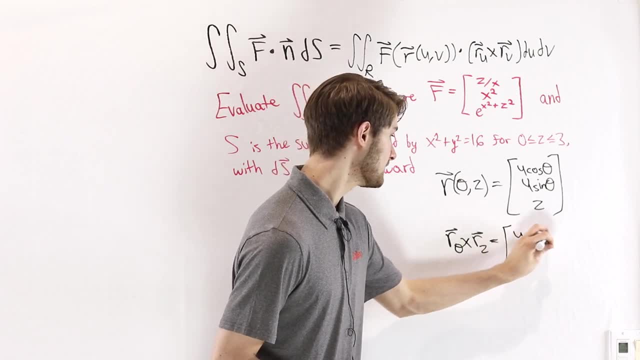 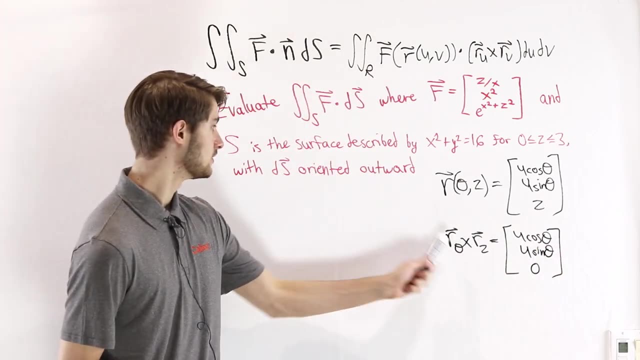 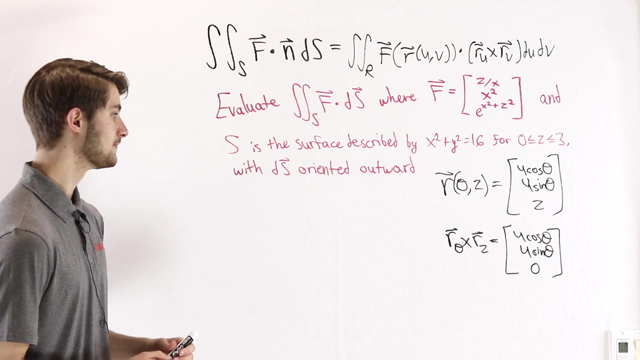 r sub z was four cosine theta, four sine theta and zero. Now is this vector oriented outward, like we want it to be? Well, let's think about what would happen if we plugged in a particular point. Say, we plugged in, theta equals zero and z equals zero. 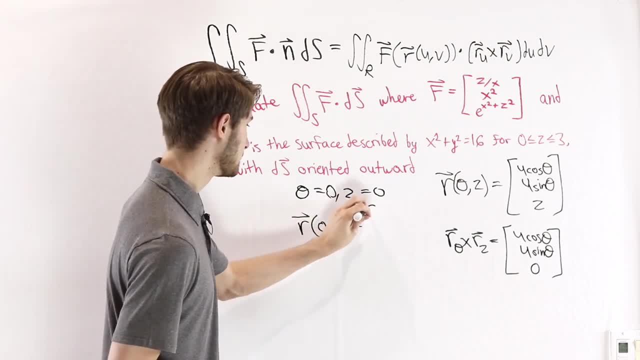 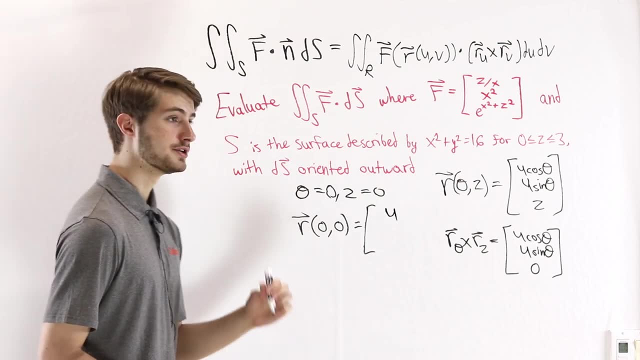 In that case we're going to have r of zero and zero, which will be four times the cosine of zero is one, so that's just four. four times the sine of zero is zero, so that's zero, and z equals zero. 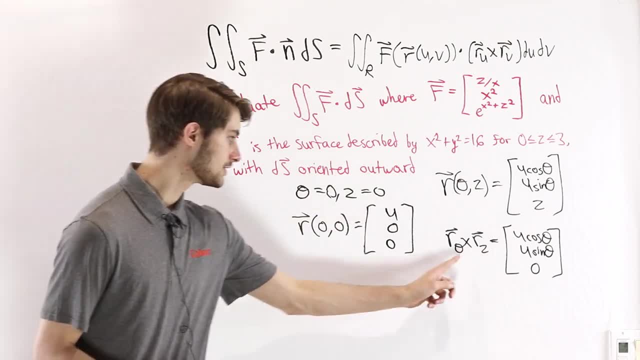 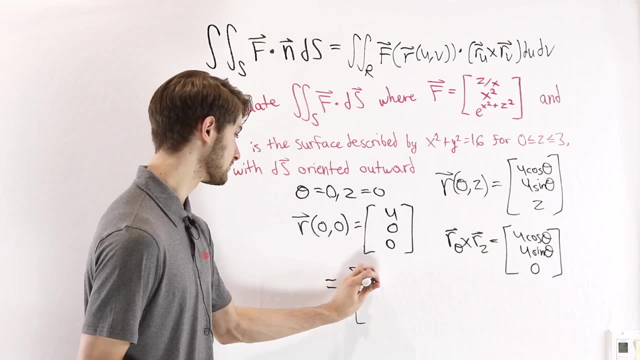 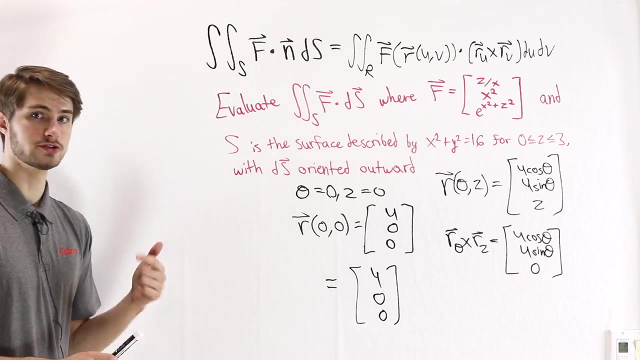 So this is our point. and then our normal vector is going to be given by this cross product evaluated at zero. zero That's going to be four cosine zero is four, four sine zero is zero, and then we have a zero. So this is the normal vector to the surface. 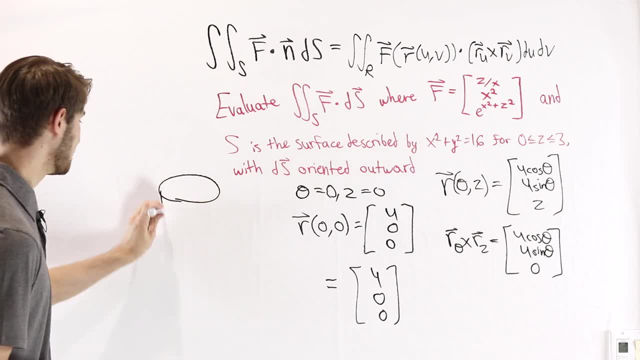 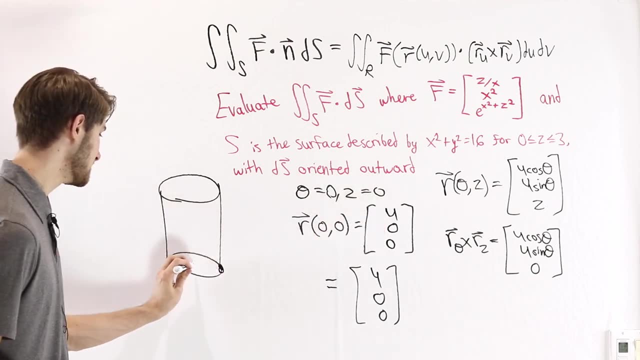 Remember that this surface is a cylinder, so we're looking at a surface that looks something like this. The point four: zero, zero is going to be at the bottom here, in the positive x direction, and the normal vector is going to point outwards. 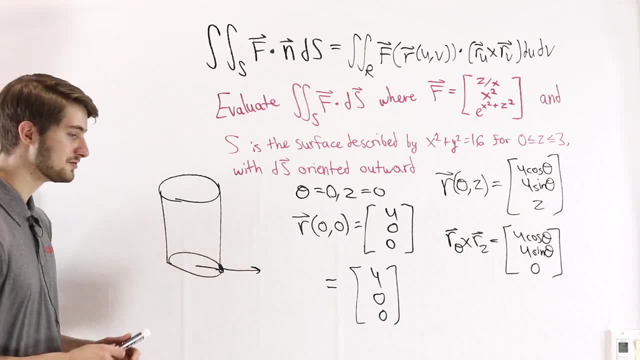 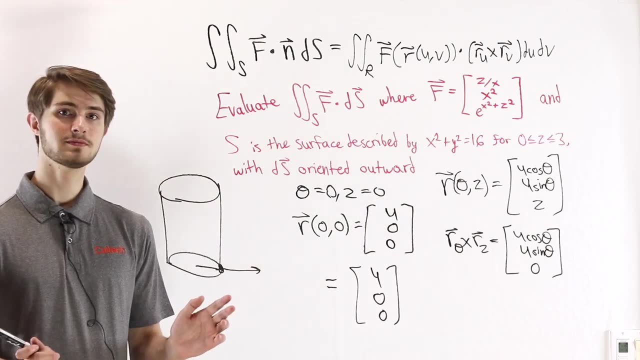 in the positive x direction, which means that this normal vector is indeed oriented outward. so this normal vector is the one that we need. We don't need to take the negative. Now, before we plug everything into the integral, let's compute the dot product of f with r: zero, zero. 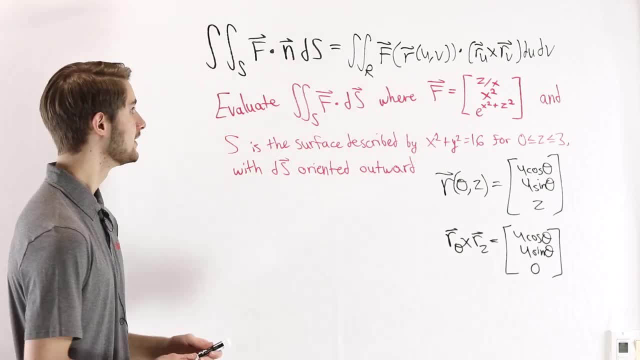 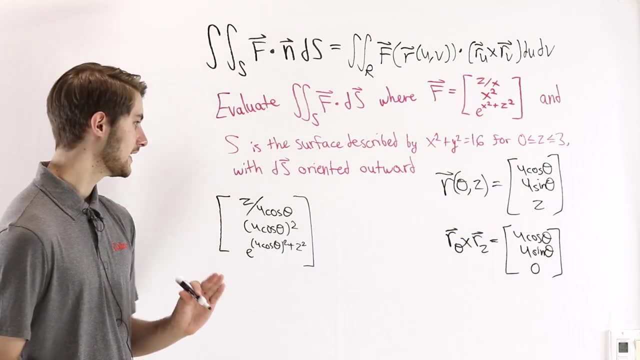 So we'll start with r sub theta cross, r sub z at the beginning. That dot product is going to be first this vector, field f. if we plug in the point here Now we dot that with the cross product that we have right here, And when we do this dot product out. 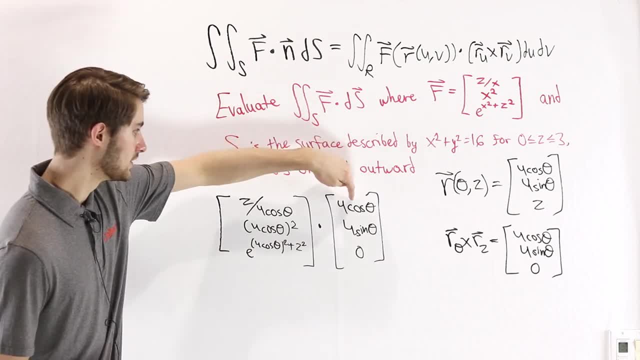 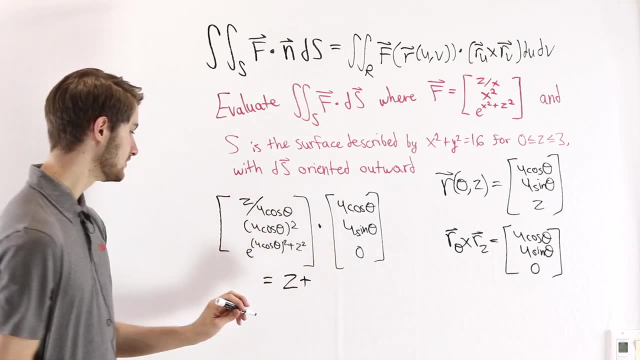 notice first that we're gonna have the x components multiplied together. The four cosine theta on the top and bottom will cancel, so we'll just have a z. Then we add the product of these two, which is going to be four squared times four, zero, zero, zero. 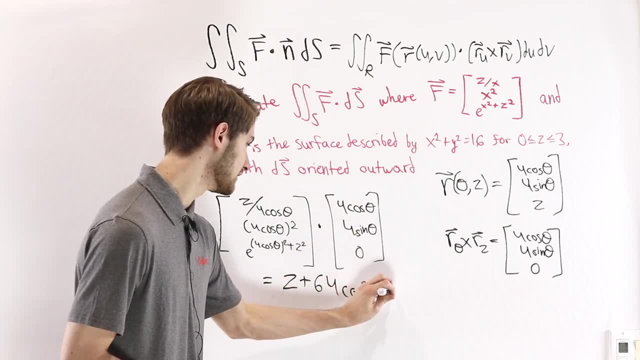 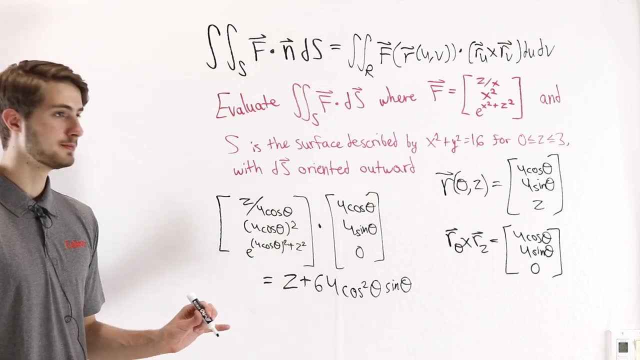 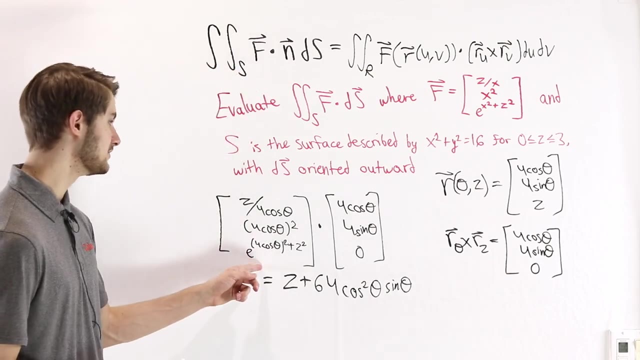 So r is 64 cosine squared, theta sine theta. And then we're gonna add e to the four cosine theta squared plus z squared, but just times zero, Because the z component of our normal vector is zero. it doesn't matter what the z component 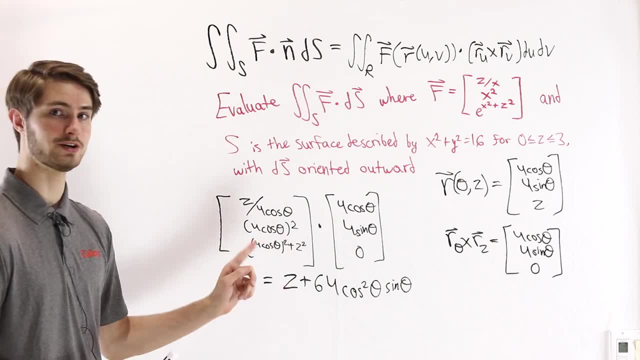 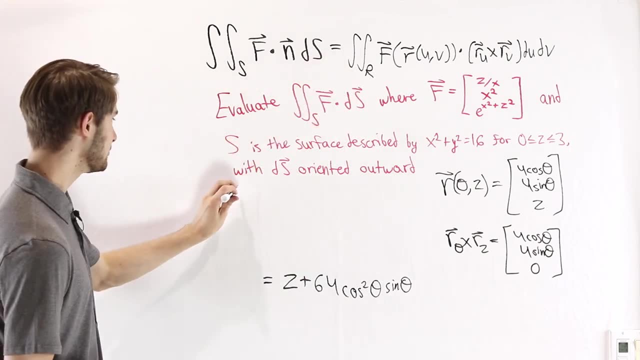 of our vector field is. That's not going to contribute to our answer at all, so we don't need to worry about it. That means that our final integral is going to be the double integral over the same ranges, as in the scalar field case. 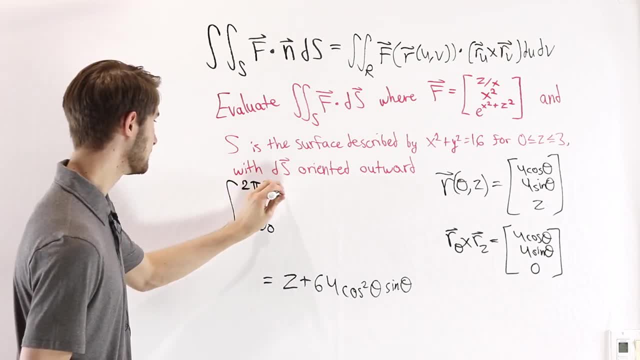 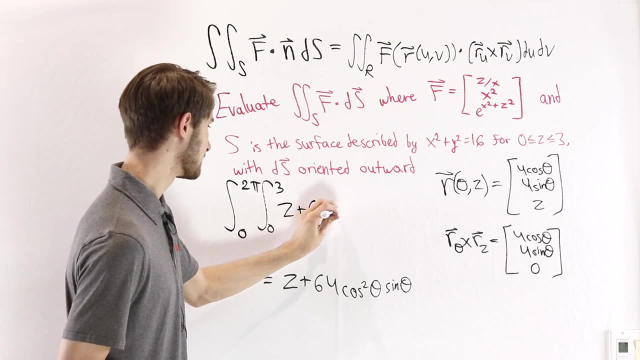 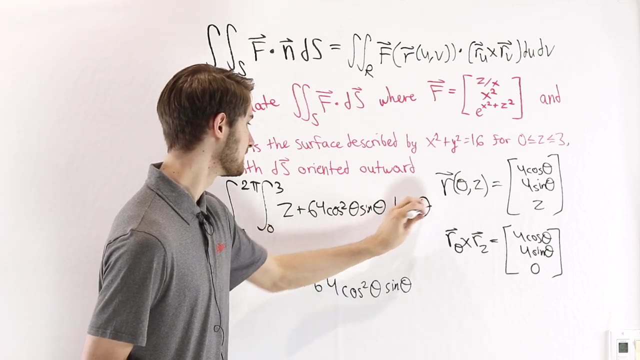 So the integral from zero to two, pi of the integral from zero to three of the dot product that we just calculated. so that's z plus 64 cosine squared theta sine, theta times dz d theta. From there it's just an ordinary double integral.